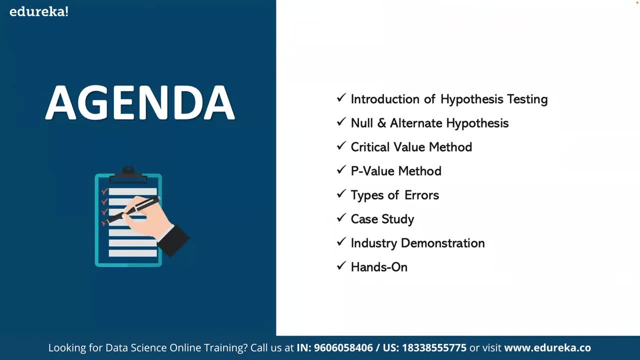 alternate hypothesis And we will look into one of the well-known methods that's called as a critical value method in performing the hypothesis testing. Then we will look into the concept of p-value method. How do we perform the hypothesis testing by referring to the 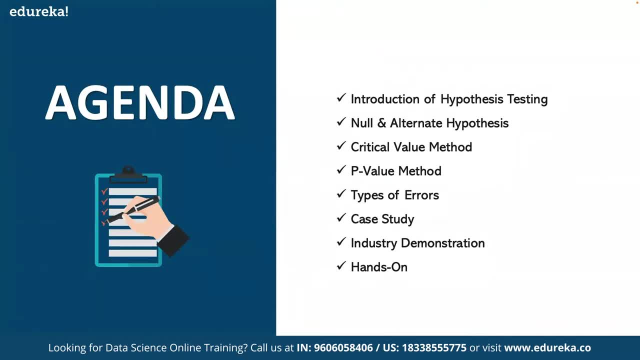 p-value. Then we will understand about the types of errors that we generally come across in statistical testing, And then we'll take up a case study and a demonstration of the scheme so that you'll get a complete picture of this hypothesis testing Now before we get started. so how many of 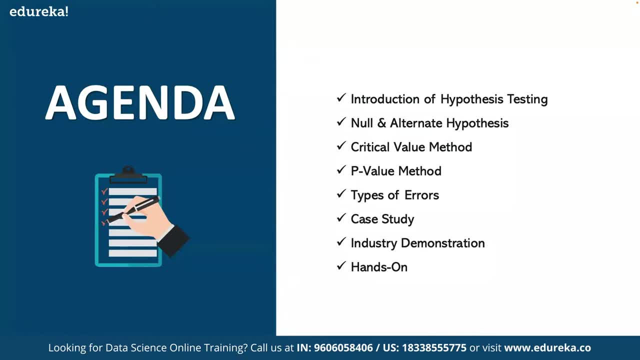 you are aware of data science and what exactly that is going to do So here when we say data science, if I want to specifically talk about this data science here, data science is all about finding the patterns in the data by analyzing the data set in an efficient manner. 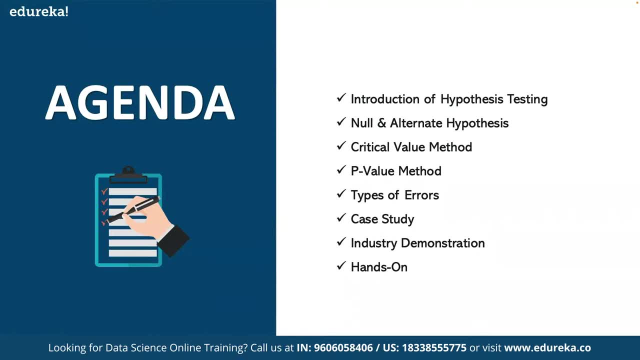 Now, while finding the pattern, we are going to apply various concepts of science. So let's take a look at some of the concepts of statistics and to validate whether my assumption is being exhibited by my model, That is when we perform this statistical hypothesis testing. So the 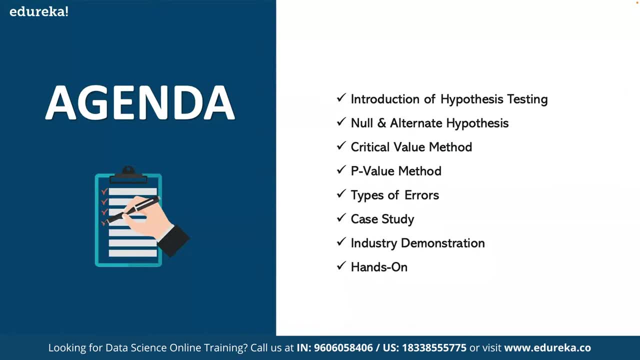 importance of this hypothesis testing is it will help us to validate whether it is a manual one or whether it is an automatic one. So that's the core idea over here. Okay, Now, as part of your learning journey in this data science, with Python certification training. 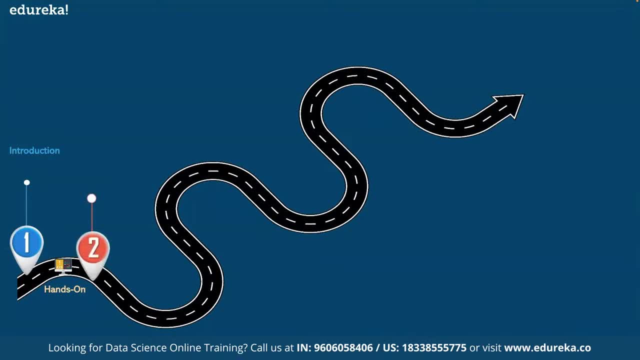 program. in the module one you'll have an introduction to Python programming language and the data science, And the module two is about working with sequences and the files. Module three is about deep dive into the functions, object-oriented programming structures, modules. 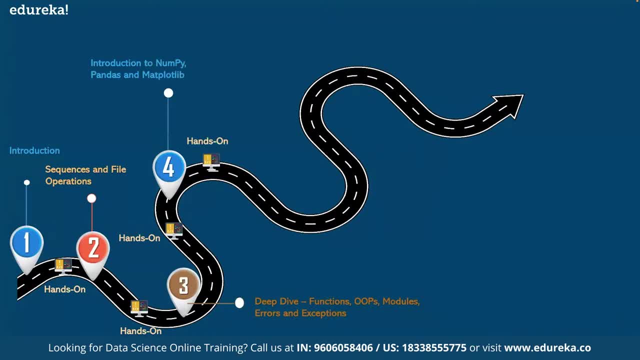 errors and exceptions. Module four is about NumPy, Pandas, Matplotlib. Module five would include the data manipulation with Pandas library. Module six is working with machine learning algorithms And learning the core basics of the machine learning algorithm, And module seven is about 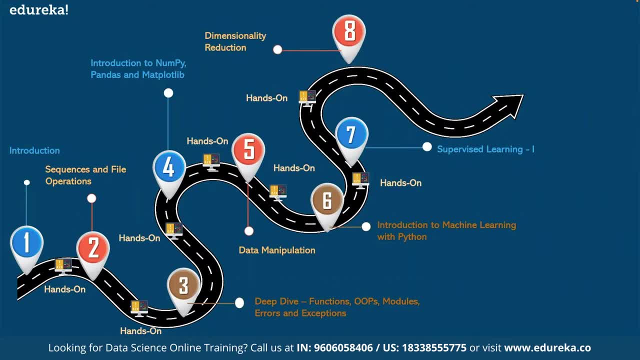 learning, the supervised machine learning, And module eight is dimensional reduction And module nine is about the unsupervised learning. Module 10 is the reinforcement learning. As you can clearly see, each and everything that is required for you to work as a data. 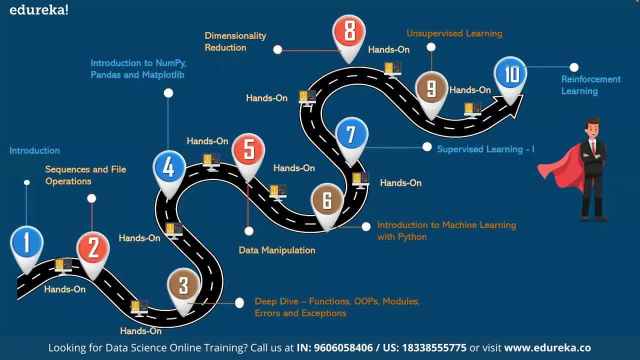 scientist and to become an industry are being covered in this data science with Python certification training program, And it follows a special learning approach that's called as a structured learning approach, which ensures that you, as a learner, will learn in a progressive manner. It doesn't matter. 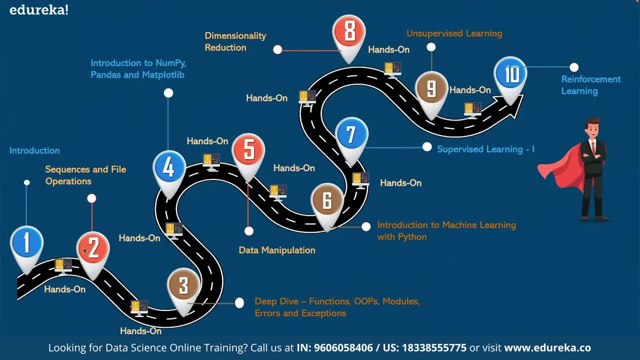 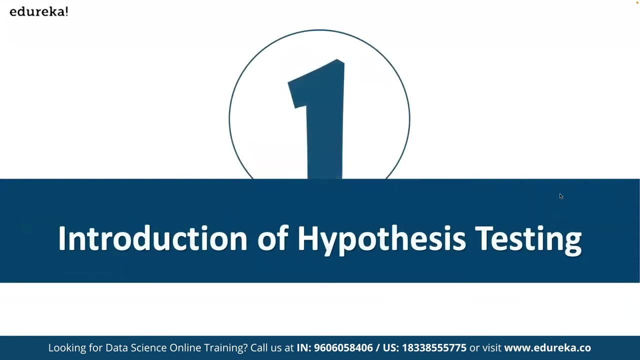 from which background you're from. Because of the curriculum design, you will be able to follow along and become an expert in understanding which technique to apply while analyzing the dataset. Okay, Now, coming back to our session's agenda. what exactly is this hypothesis testing? 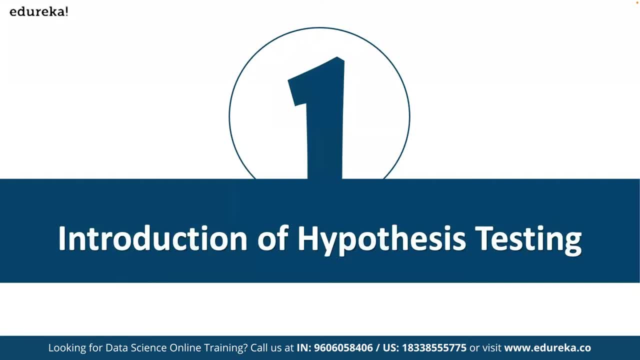 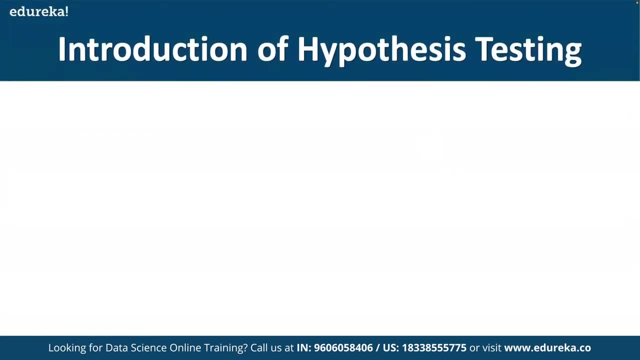 Now when I talk about hypothesis testing, hypothesis testing is a statistical analysis. Here we are going to put our assumptions about a population parameter to a given test. Now we use it to estimate the relationship between two variables. Okay, Let's take up an example. 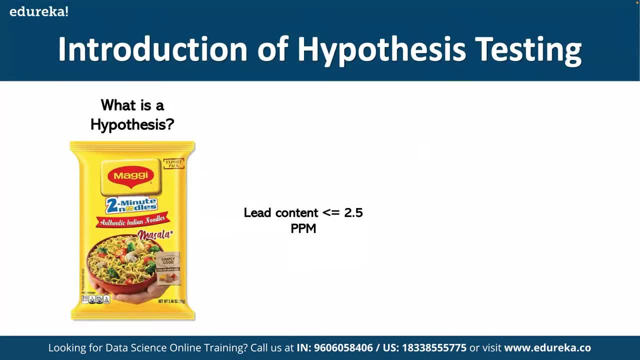 So we assume that, okay, for a Maggie noodles. Okay, So we assume that for a Maggie noodles, there is a lead content of less than or equal to 2.5 PPM. Now, this is my assumption, Okay, Now, what I'm going to do is so, if you think about the production of Maggie noodles by 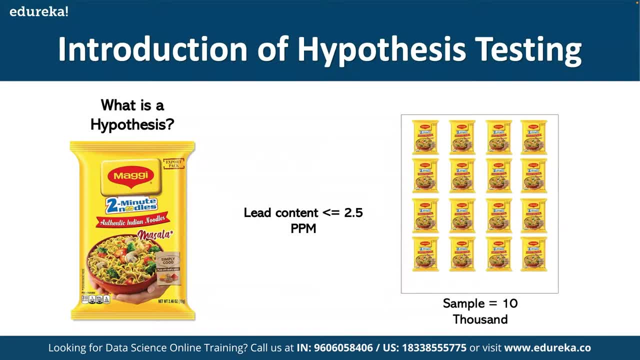 a Nestle company. they will be producing the lacks and lacks of products. Now think about testing lacks and lacks of products every day. that is going through each and every product and testing it. So obviously you cannot test each and every Maggie product which is being 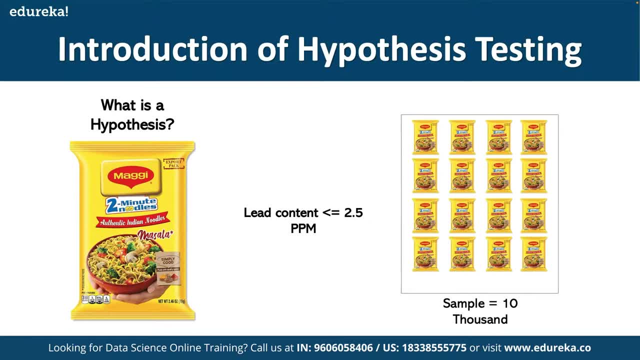 produced by the Nestle company because one you will be using entire stock in your testing. It will be lost for the business And even it's not a recommended one. Think about 10 lakhs of Maggie packets that you have to test it. how much time it will take, So obviously. 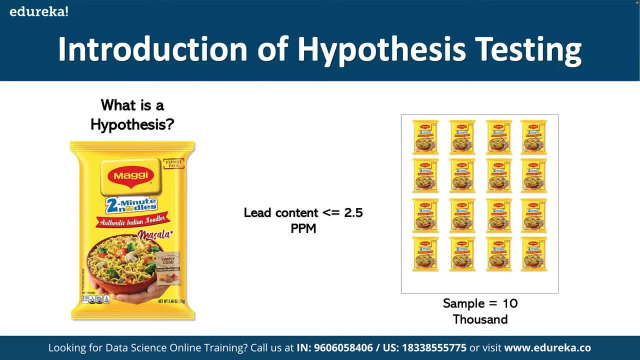 we cannot test each and every Maggie product, So what I'm going to do is I'm going to pick up a sample, maybe out of 10 lakh products, which has been prepared by the Nestle company. I'm going to pick up 10,000 products. 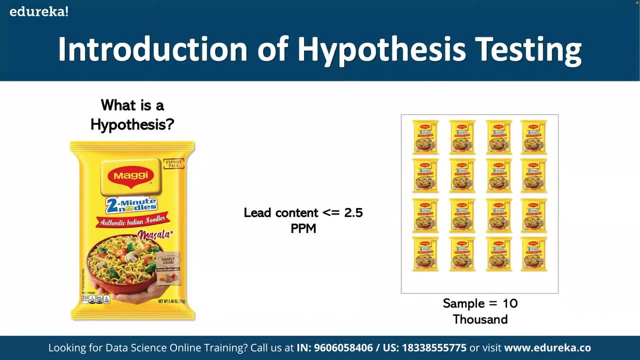 Okay. So what I'm going to do is I'm going to pick up a sample, maybe out of 10,000 products. so 10 lakh product is the population, And from that population I'm going to select a sample. in this example, that is 10,000.. So once I select the sample of 10,000, then okay. 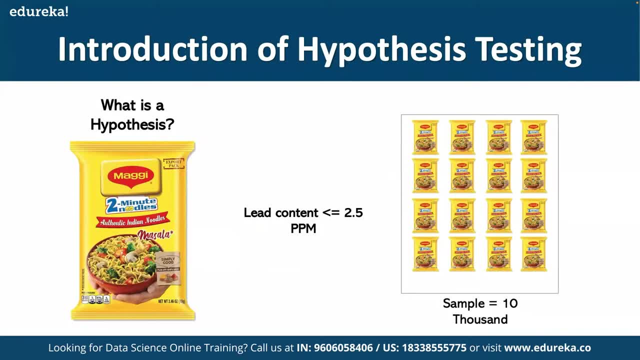 then I'll go ahead and perform the analysis on this 10,000 packets. So what it means is, once I like, instead of testing on the 10 lakh products, I'm testing on 10,000 products, and whatever the outcome that I'll get, I'm going to generalize it for my entire population. 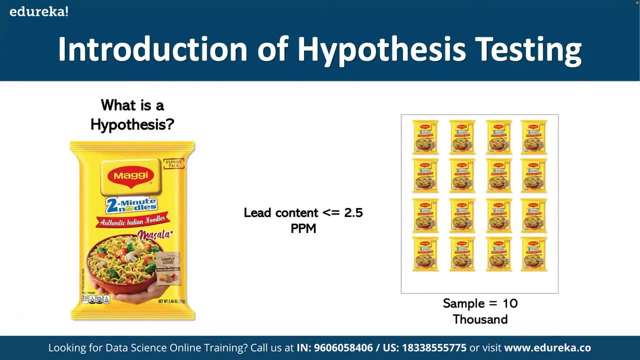 Let's say, out of 10,000 packets that I've sold, So I found that all the packets is having the lead content of less than 2.5. Then I will report that, okay, the Maggie is safe and the lead content is less than 2.5.. Okay, That is the overall way in which that we are. 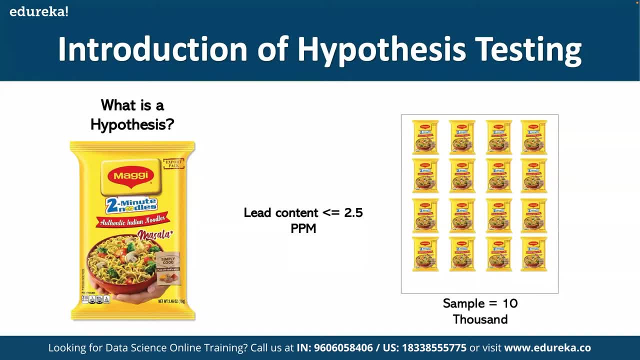 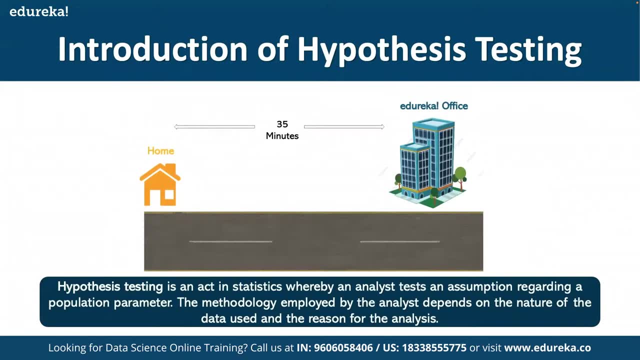 going to interpret this scenario. Okay, So that is how we are going to interpret the same Here when we talk about the hypothesis testing. so hypothesis testing is an act in statistics where an analyst tests an assumption regarding a population parameter. In the previous example, 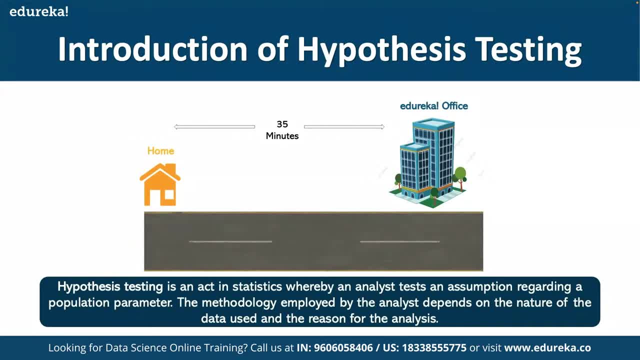 here the population parameter is actually my lead content in the Maggie noodles, which is produced by a Nestle company, So that we are going to test that assumption. okay, for the population parameter And this methodology employed by the analyst depends on the nature of the data and the reason. 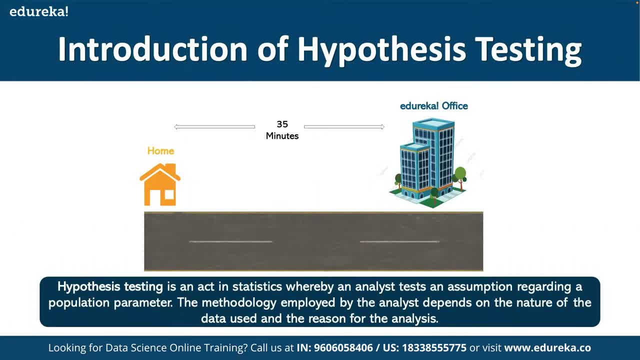 for that analysis. Okay, So that's the overall idea. So if I want to give you some more examples of statistical hypothesis. so hypothesis is nothing but the assumption. Maybe we've got a teacher or we've got a lecturer. A lecturer assumes that 60% of their college students come. 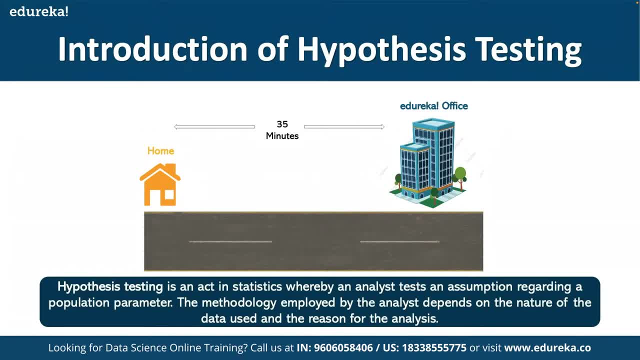 from, let's say, like higher middle class family. So these are all just the statements. or people who smokes, they are more productive. or women use more social media than men. So these are all some of the assumptions that we have. So once we have this assumption, we call this. 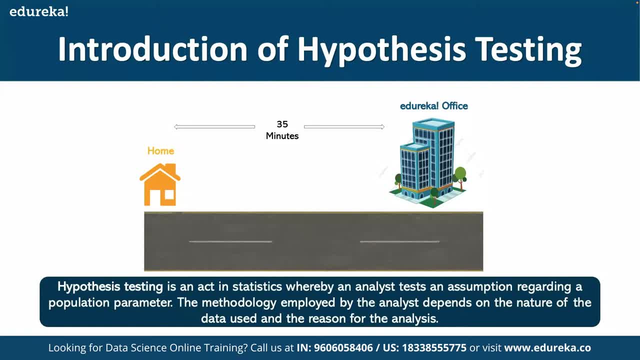 as hypothesis And we are going to test this hypothesis. In order to test this hypothesis- that is our assumption- we are going to select a sample from the population and then perform the testing Here. The reason why we use it to test it always depends on the nature of data and the reason. 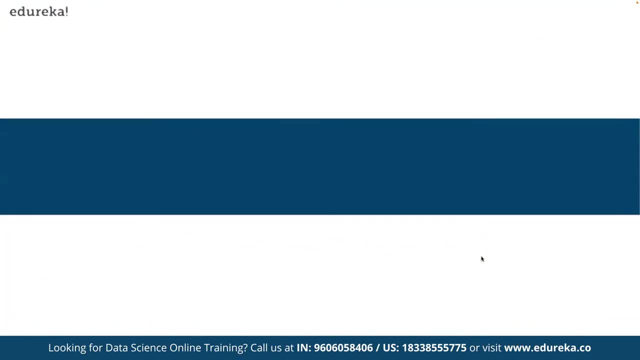 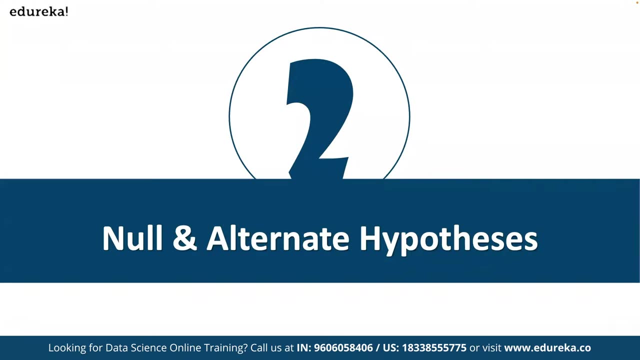 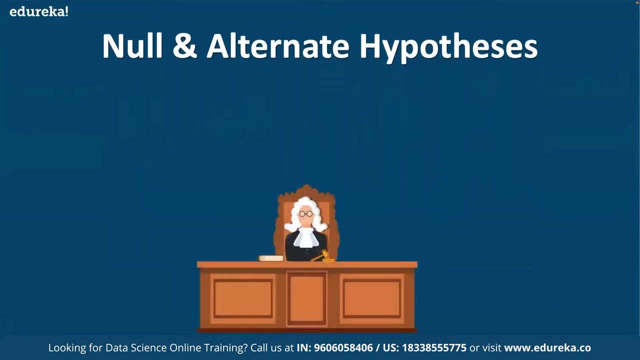 for that analysis. So that's the core idea about this hypothesis testing. Now, while performing this hypothesis testing, so we have null and alternate hypothesis. So here the null hypothesis is the assumption that the event will not occur. Okay, It's a, it's something that the 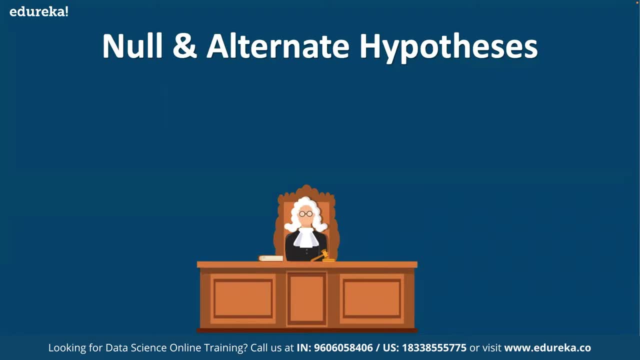 event will not occur. So a null hypothesis has no bearing on the study's outcome unless it is rejected, And we have something called as alternate hypothesis. Alternate hypothesis is a logically opposite statement of my null hypothesis. So if I accept the alternate hypothesis, it means I have rejected a null. 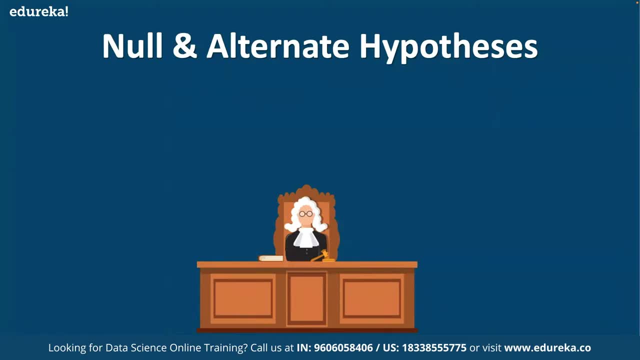 hypothesis, To give you an example, I have mentioned that smokers make more sale than men, or non-smokers- Okay. Or vegetarians miss few flights- Okay. Or vegetarians miss few flights- Okay. Or vegetarians miss few flights, Okay. Or 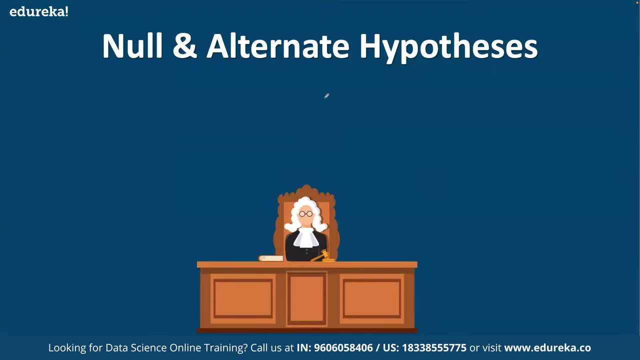 Creating flies. Okay, Let's do one thing. let's take up a hypothesis: Okay, Vegetarians miss few flies. Okay, Not those many flies. Okay, Didn't have any flight. Okay, That's not a real question about flying, flying. 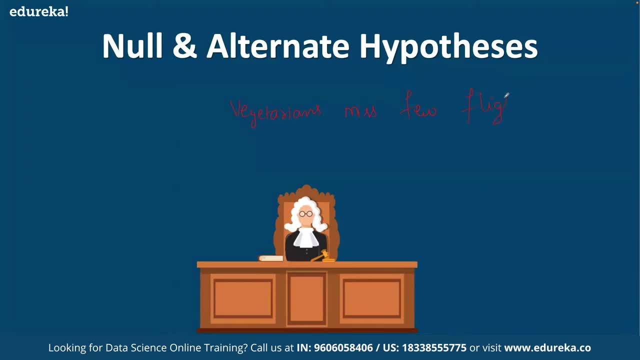 Okay, Hum, אבל I gotta to finish the concept of the question. let's finalize the question quick. Okay, Not all flies must stay inside. Okay, For the first time, if we run as we do, the Goodnight Test, the procedure will give. 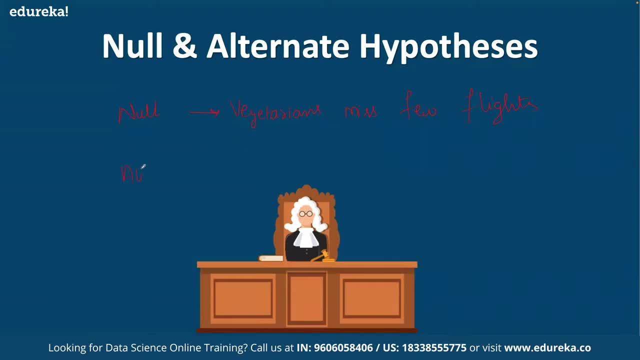 the expectation that animals will not get through with no flight flights. So we are going to have an alternate hypothesis. In this alternate hypothesis, what we would say is: it will be logically opposite to what we see. So logically opposite can be something as okay, which day, like vegetarians, miss more flights, So that can be a logically 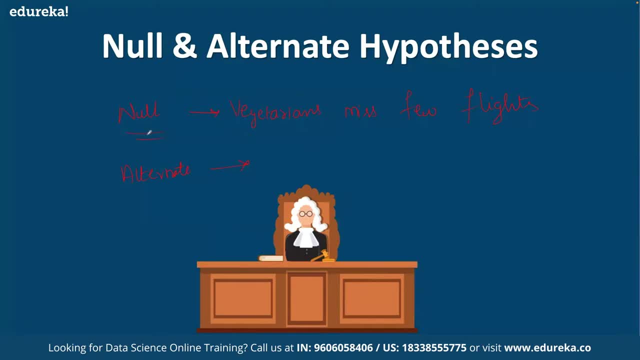 opposite statement. So null hypothesis is the current assumption and the alternate hypothesis will be the logical opposite statement of the null hypothesis. And we will perform the hypothesis testing, whether to validate whether whether the null hypothesis is correct or whether the data that we have got follows the current belief or whether it follows the 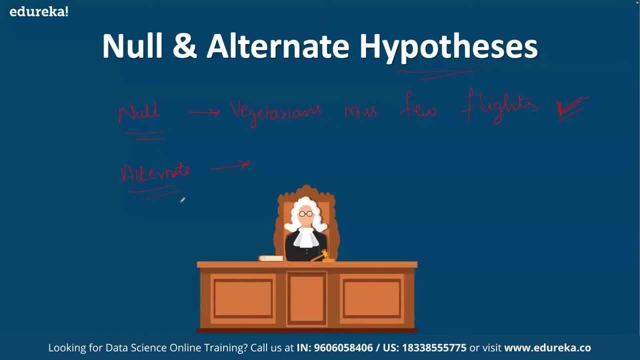 alternate belief. So that's the overall idea in the scenario team. That's the importance of null hypothesis and the alternate hypothesis. Now that you have the basic understanding of this, Now we will see the general idea of null hypothesis and the alternate hypothesis. So let's proceed. 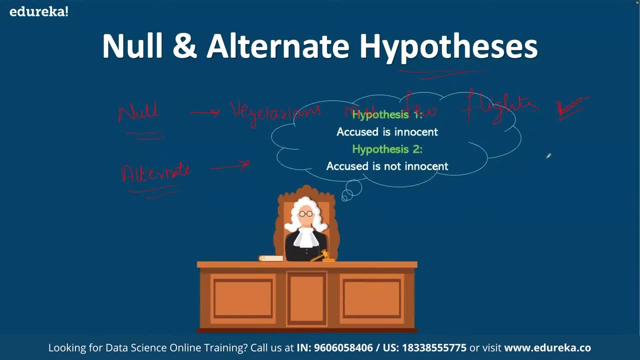 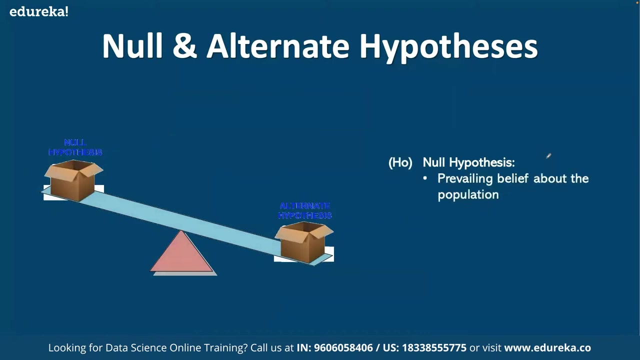 ahead. This is another example where I've got a hypothesis where hypothesis 1,, which is my null hypothesis- says that accused isn't is innocent and the logically opposite statement is the alternate hypothesis, where the accused is not innocent. Okay, So that is the overall idea about null hypothesis and the alternate hypothesis. We 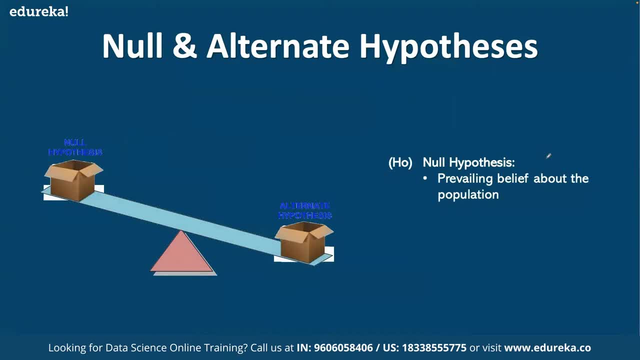 the null hypothesis, which the which, with the help of the symbol h0 or the null hypothesis, so null hypothesis refers to the existing belief about a population. so we assume that the status quo is actually true. that's our assumption, and we have something called as h1. we represent this h1. 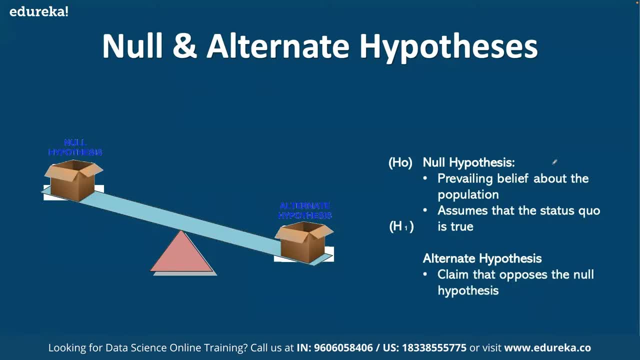 with alternate hypothesis. now, this is a logically opposite statement of my null hypothesis in this scenario. so we are going to check the overall condition. so what we will do is we are going to consider the given statement and we'll perform the testing to validate whether it follows. 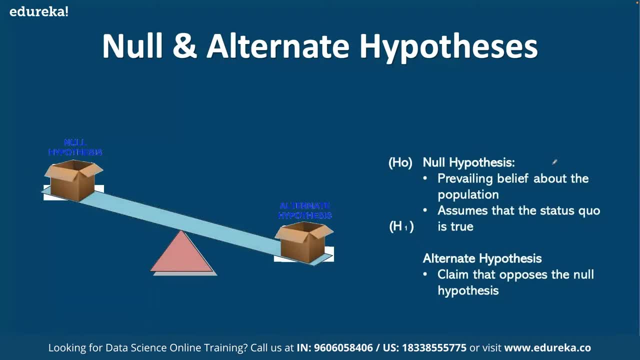 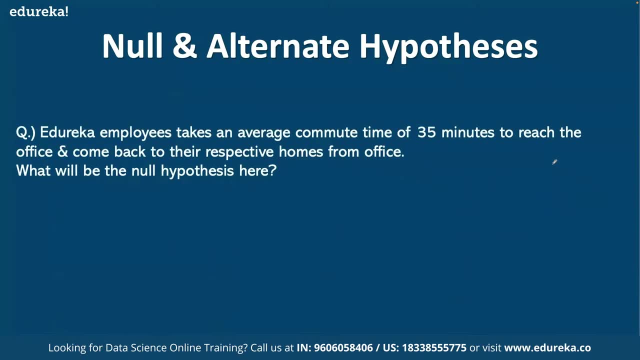 the null hypothesis or the alternate hypothesis. okay, so now that you have understood about what exactly is this null hypothesis and the alternate hypothesis, let's take up a question to get a clear picture about the same. so here we've got a question that says that edureka employees takes an average commute time. 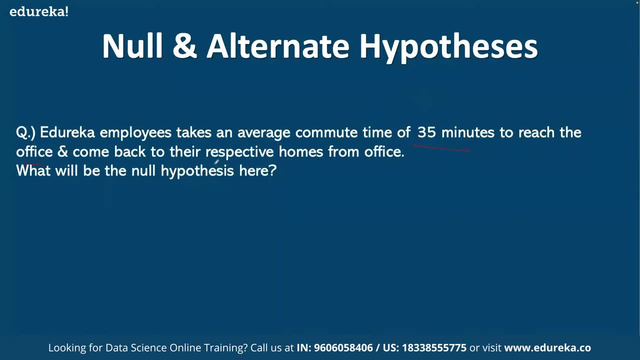 of 35 minutes to reach the office and come back to their respective respective homes from office. now, in this scenario, what exactly is the null hypothesis? so, in this example, the null hypothesis is the one which is our current belief, which is nothing but edureka team or the employees. 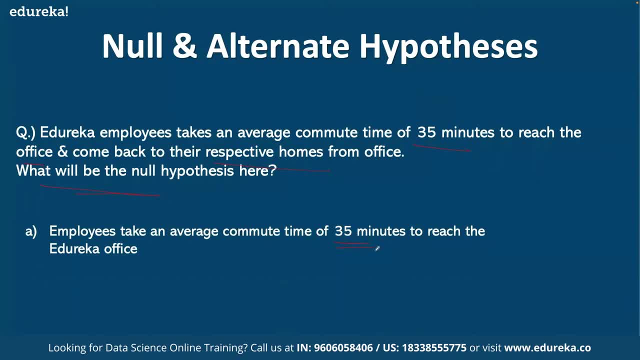 take an average commute time of 35 minutes to reach the office and come back to their respective homes from the office. okay, so that's my null hypothesis, and my alternate hypothesis is the logically opposite statement, which says that edureka employees takes more than 35 minutes on. 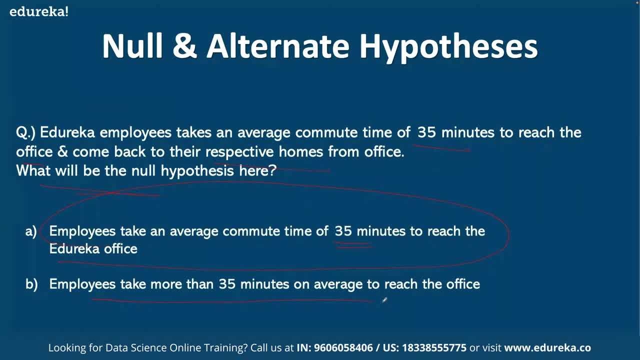 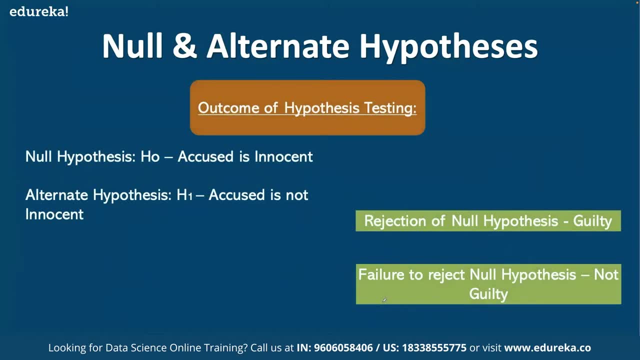 an average to reach the office. so that is the first step. we define our null hypothesis and the alternate hypothesis. so if the null hypothesis holds good, then our current belief holds good. maybe the current null hypothesis is accused is innocent. so that's my current null hypothesis, if the data follows else. 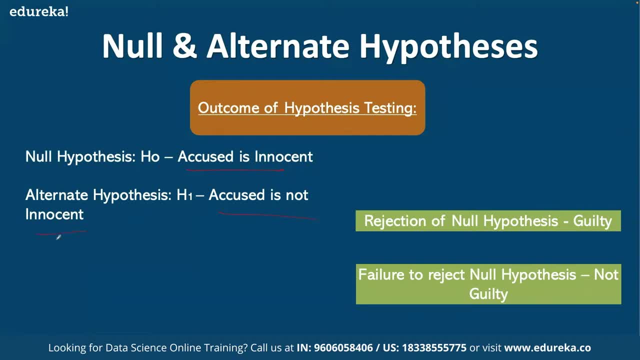 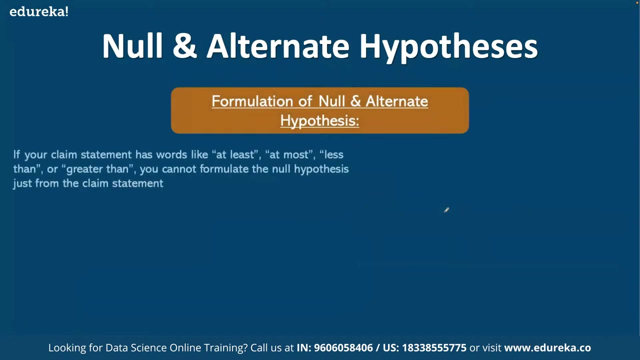 it will follow the alternate hypothesis which says that accused is not innocent. okay, so in this way we are going to specify, specify the same next here, in this scenario. so, if i go ahead with the alternate hypothesis, we are going to reject the null hypothesis. so here, when we are formulating this null hypothesis and the alternate hypothesis, suppose, 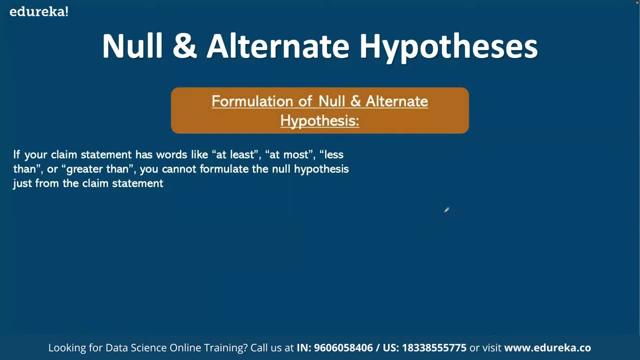 if your claim statement has the words like: at least, at most, less than or greater than then in such scenarios you cannot formulate the null hypothesis just from that claim statement. so what you have to do is you have to create something like this: okay, so the rule to formulate the null and alternate hypothesis is: 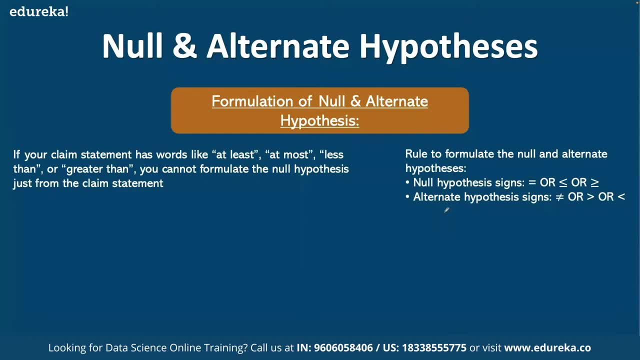 like this. so, if you like, it's like equal to, greater than or equal to, or less than or equal to. so these are the ways in which you are going to formulate your null hypothesis and the alternate hypothesis is the opposite of it. let's say, if i'm using equal to, it is like all not equal to if it. 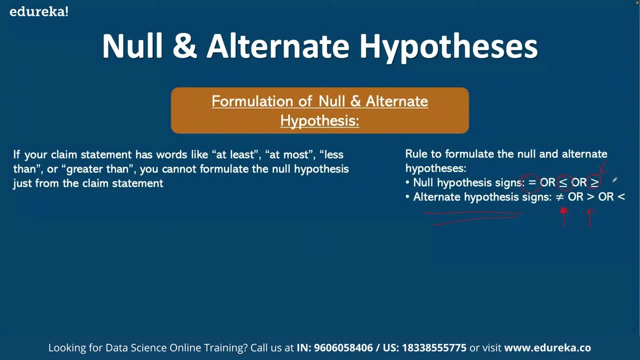 is less than or equal to, then it will be greater than. if it is less than or equal to, then it will be greater than or equal to it, then it will be less than. so this is how we are going to formulate the null hypothesis and the alternate hypothesis. okay, once we formulate this null hypothesis and 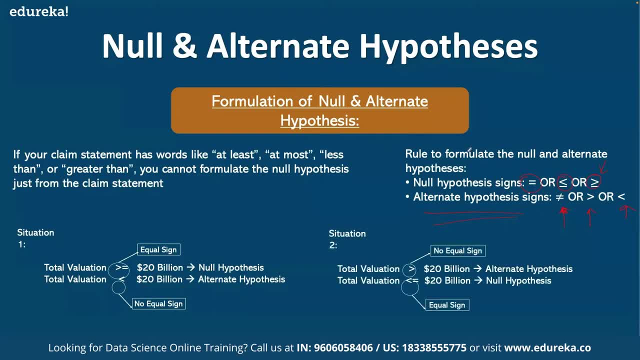 the alternate hypothesis, then we will go ahead and perform the testing now. in this example, i have made use of greater than or equal to sign. hence okay in my alternate hypothesis. i've got less than so in my null hypothesis. uh, in in this scenario, okay, i think. 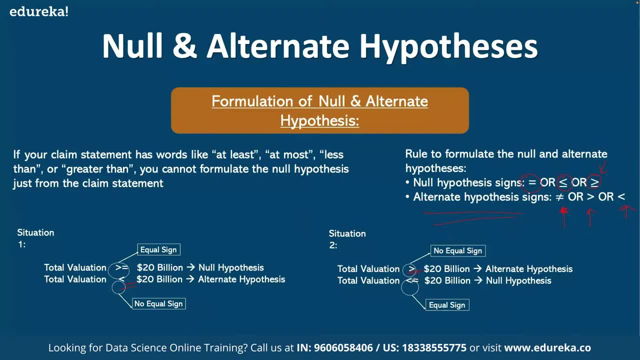 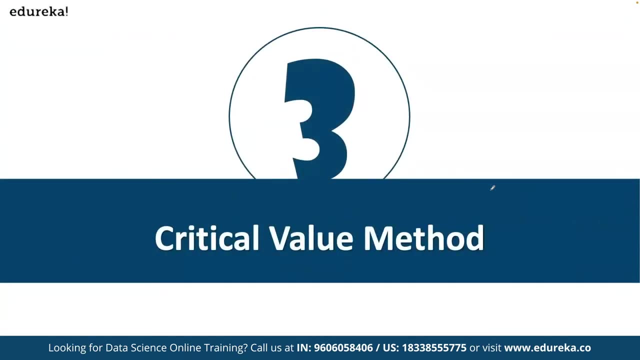 on. yeah, if you observe, i've got a greater than and hence, in the below one, i've got less than or equal to. so that's the overall way in which that we are going to formulate the null and the alternate hypothesis. now that you have understood about null hypothesis and the alternate hypothesis. 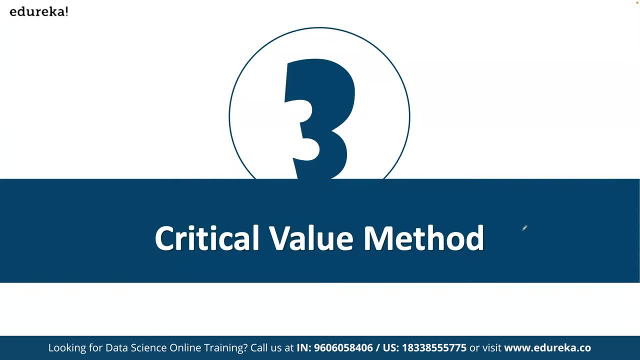 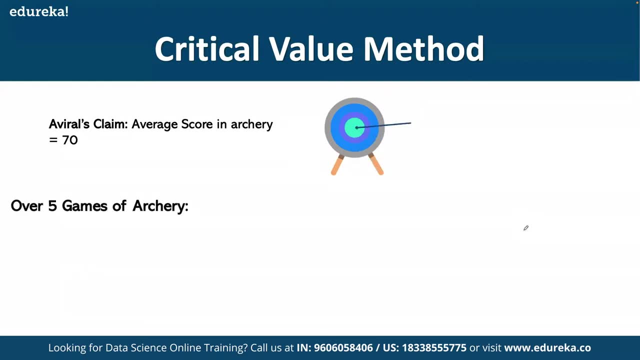 now let's understand about. what does it mean? by a critical value method? let's take up a scenario. so we've got a viral and evaril's claim is: average accuracy in archery is 70.. now, over the five games of archery, this is how the data is. so the average score is 20.. so if i've got, the average score is 20. 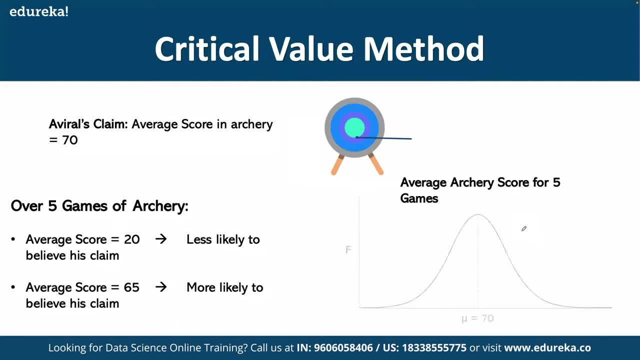 then it is less likely to believe this game claim and average score is 65, it is more likely to believe claim is more likely to believe claim because average score is 20. then when we use data disable Type lamenter system says average score is 70. then it's not less likely to believe every claim for every. 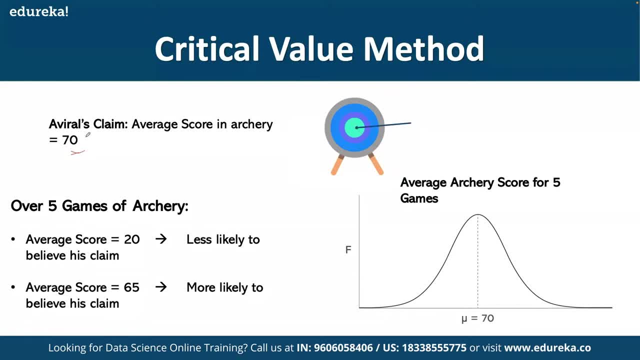 this is much closer to the value of 70. so we have got a claim that is 70 now, with the average score as 70. now if i, if i'm saying that average score is 65, then it is more likely to believe because we've got the detail, or we've got the information that the value is 70, so which is uh, and the 65. 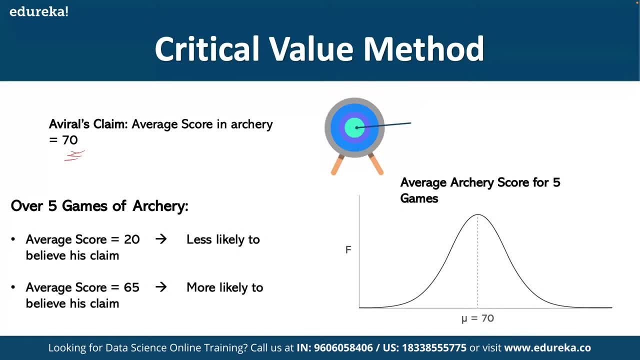 that we have got. so it is closer. okay, so the 65 that we have got is closer to 70, hence this is more likely to believe the claim. so in this way, so we'll get the value. so in this example the mean is 70. okay, and let's suppose, if my value is 50, so like we have in order to ensure that, okay. 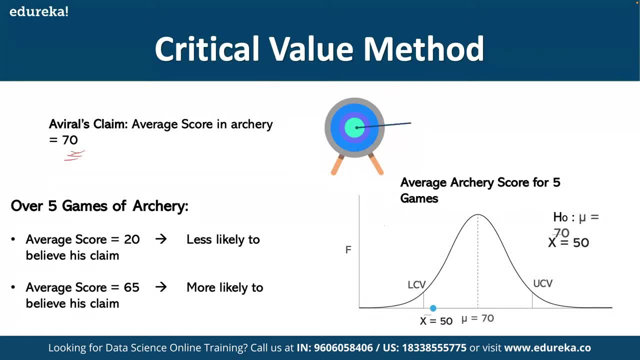 whether it's whether it holds good or whether it's holds uh, whether it does not hold good or not. we are going to look into the confidence values. okay, on the left hand side you can see the lower confidence value and on the right hand side you would observe the upper confidence value. so we will check whether it. 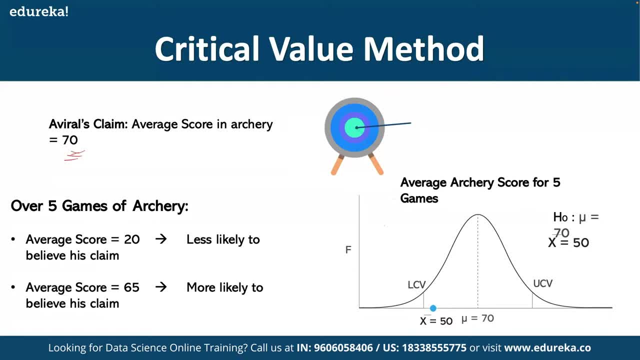 it is present in that confidence value or the confidence region. okay, now, based on the values that we have got, so then we are going to where exactly the value would lie. okay, so we are going to look at the confidence value and we are going to look at the confidence. 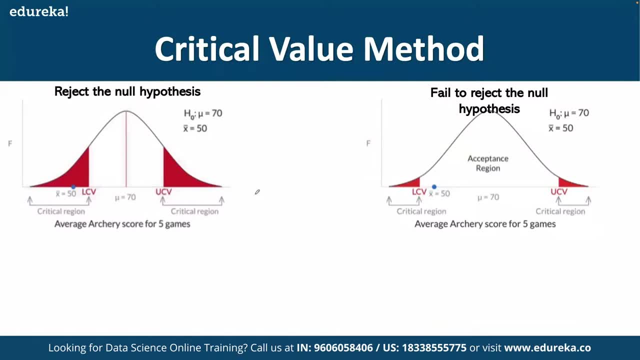 whether it lies in the lower, less than lower confidence region or greater than upper confidence region. so if we, if we get in that specific scenario, okay, in such scenarios, so we are going to fail to reject the null hypothesis. so in this example, so we fail to reject the null hypothesis. 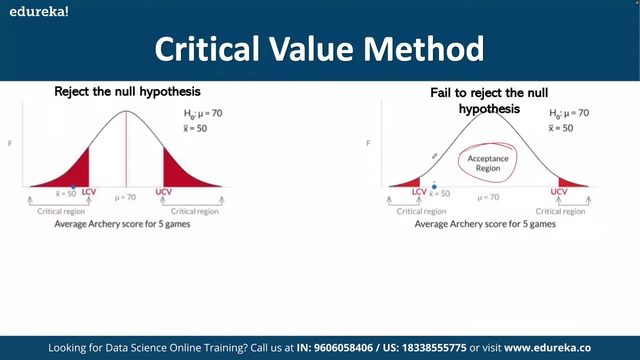 because it is present in my acceptance region. okay, if i have any value which is in the acceptance region, then in such scenarios we fail to reject the null hypothesis. so if i've got any value which is greater than uh, like which, which appears in that red region, i would say that's the region where we would say that we are. 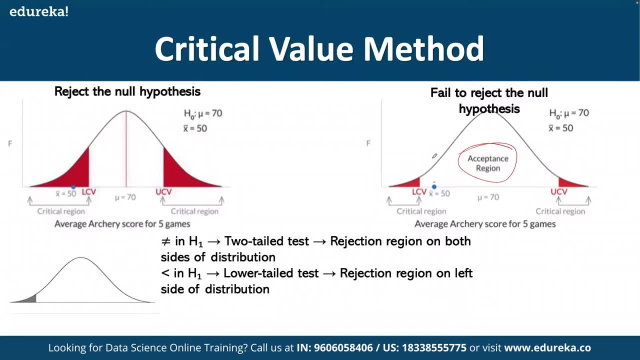 going to reject the null hypothesis and we follow the alternate hypothesis. okay, that's the overall idea in this scenario. now, in case, if you are, if you are working on two tail test, so the rejection region on both the side of the null hypothesis and the opposite side of the null hypothesis. 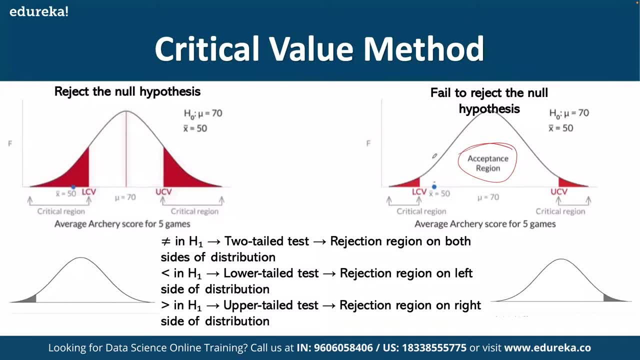 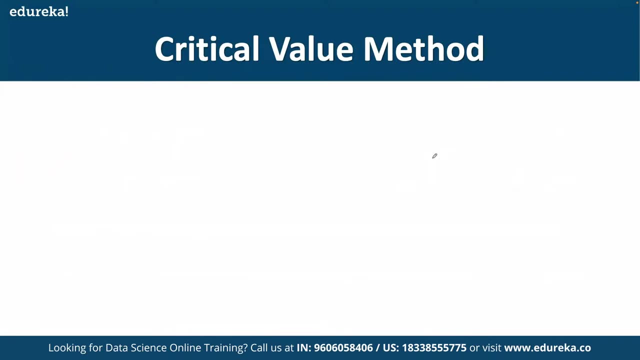 of distribution now in the. if i'm performing the lower tail test, then in such scenarios the rejection region on the left side of the distribution and if i'm performing the upper tail test, then in that scenario the rejection region is on the right side of the distribution. 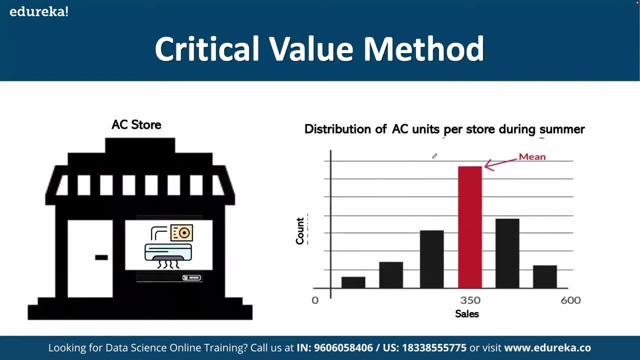 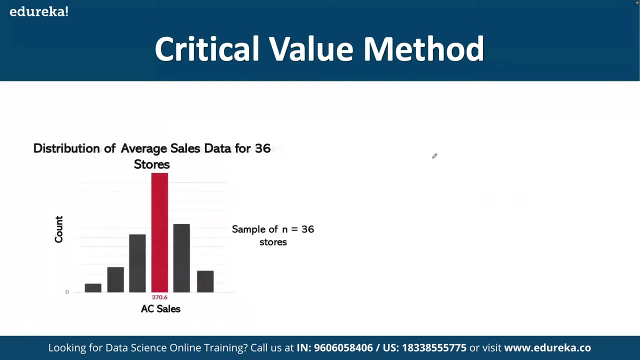 now let's take up an example here. we have got a ac store, okay, and this data over here describes the distribution of ac units per store during the summer. now, this is the information that we have got, that is, the distribution of ac units per store during the summer. now, in this scenario, okay, so let's say we've got the sample. 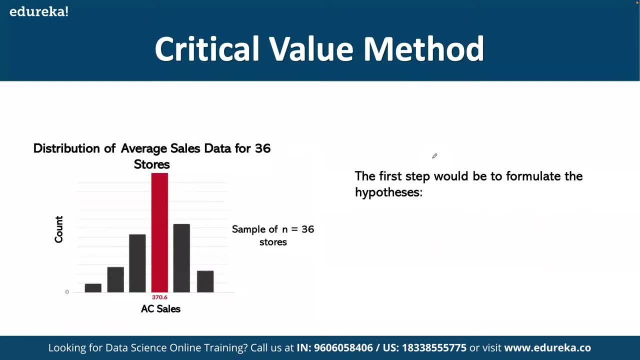 of 36 store. then what we do is: the first step is to formulate the hypothesis. so we'll define, uh, the null hypothesis and the alternate hypothesis. so the null hypothesis is 350, which means that there is no change in stored status quo, and the alternate hypothesis is the one which says that average is not equal to 350. 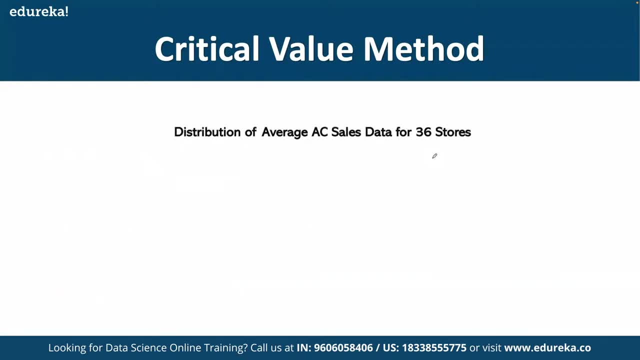 now, once we define the hypothesis, then we are going to select the sample in the scenario we'll look into the sample of 36 store. so in that scenario the sample mean can vary very far from 350. then in such scenario we are going to select the sample of 36 store and we are going to 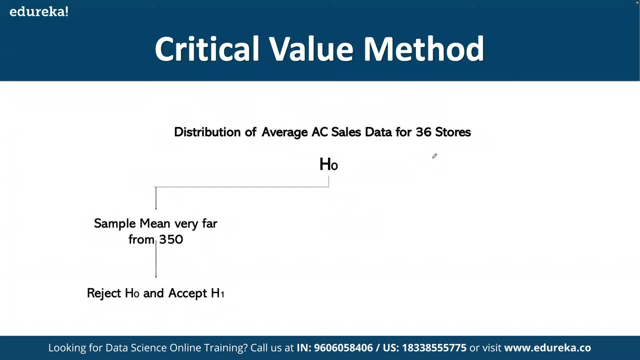 reject the null hypothesis and we are going to accept the alternate hypothesis. on the other hand, if i've got a sample mean closer to 350, then in such scenarios we do not reject the alternate null hypothesis, we just proceed with the null hypothesis itself. so that is. 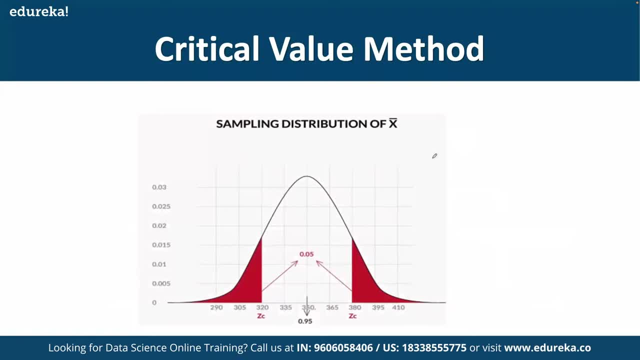 how we will make use of the critical value and then a performance of the null hypothesis from the analysis. so in this scenario, so we've got a mean and then i'm going to calculate the sample standard deviation, okay, which is given by sigma divided by square root of n. 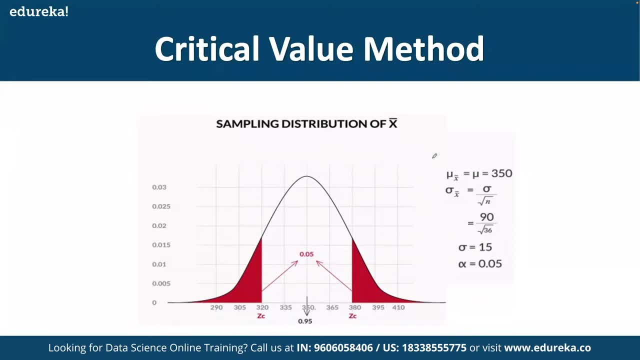 that is the number of rows that i've got and from there we are going to calculate the values. okay, and here this describes about the sampling distribution of x. so once i have the value of sigma, so i'll check on the upper confidence value and based on that, very like, based on this, so where? 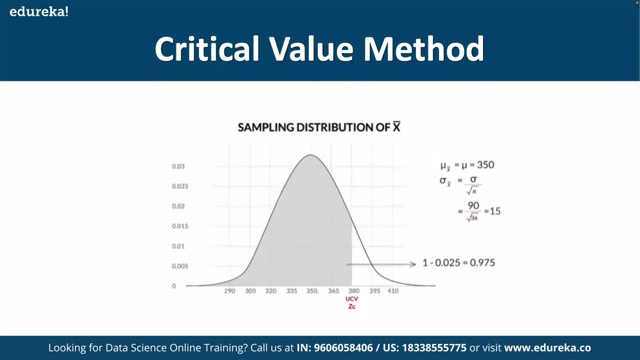 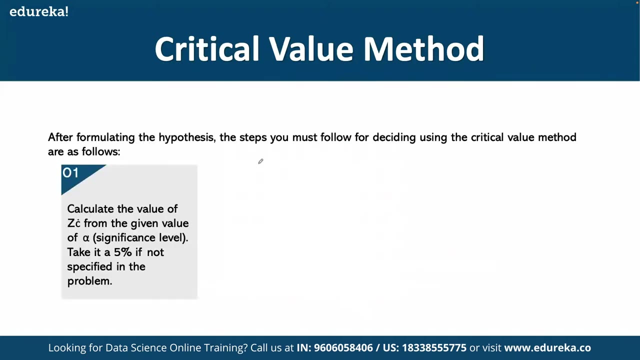 depending on where my data points would lie, i would decide whether to follow the null hypothesis or the alternate hypothesis. okay, so that's the overall idea of this critical value method. now, here, once we formulate the hypothesis, the steps that we would generally take in order to follow- uh, like the steps that we generally take using this critical value method- is: 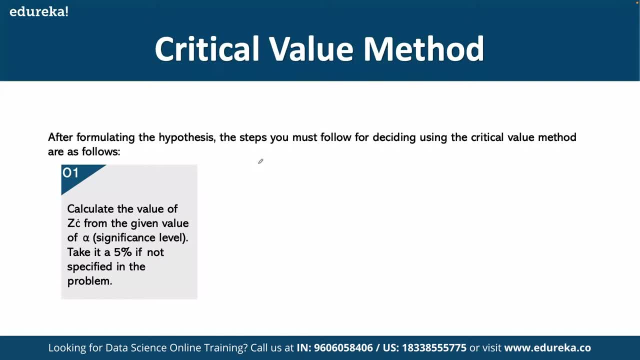 first, we are going to calculate the value of z from the given data set at a specific significance level. okay, it will be alpha, so like, let's say, it can be five percent. okay, now, once we specified the same, the next thing that we are going to do is: here we are going to calculate the critical value. 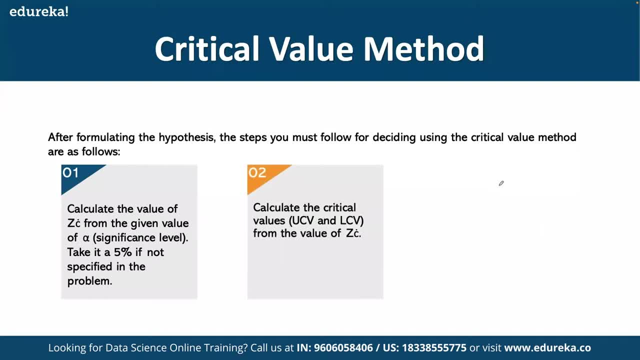 of z with respect to the critical values, that is, upper confidence value and the lower confidence value from the value of z. now, once we calculate the critical values from the value of zc, so we'll make a decision on the basis of the sample value, mean, sample mean x with respect to the critical. 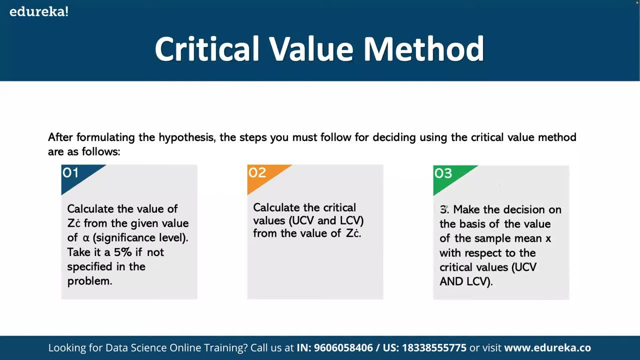 values and the lower value, zc, so we chook values. that is so with all these values we are going to decide automation based on the amount our district value巨 양 forces, that the value will axle value. then we can take theástile on下面. 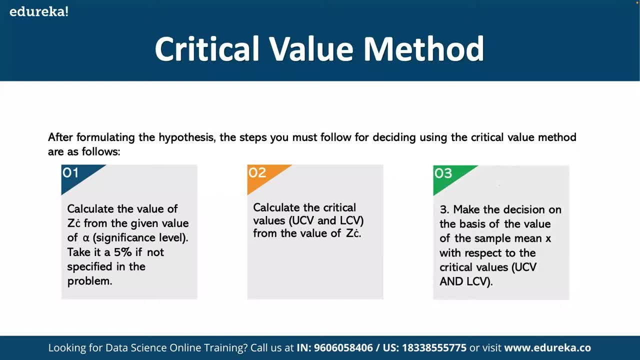 to the other direction. on장님 nonsense. z value champion, the critical value willcなたGE Upwork out hypothesis or whether it follows the alternate hypothesis. so this is called as a critical method. next, we have something called as a p-value method. now, in this p-value method, so what we will do is: 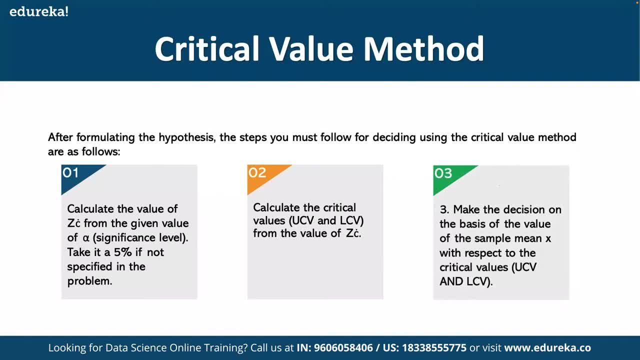 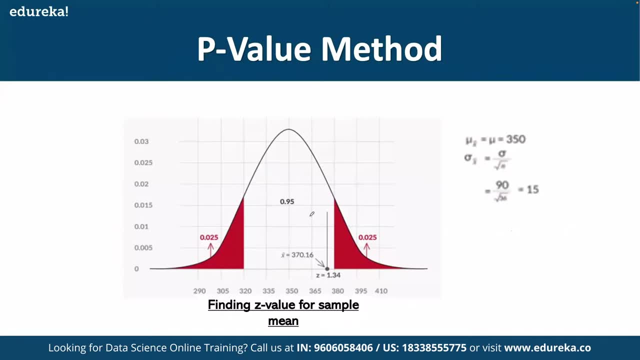 we are going to check the value of p. okay, we are going to check the value of p now in the scenario of p-value method. first, we'll find the z value for the sample. mean now, once i find the value of z, the next thing that we are going to do is we are going to 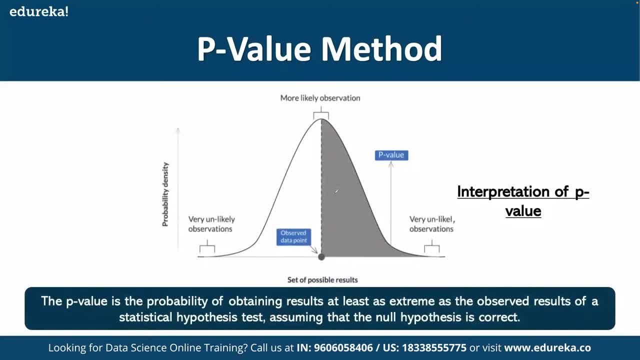 get the respective p-value now depending on value of p. so this p-value describes the probability of obtaining the result at least as extremes as observed. okay, so here like it's the probability of obtaining the results at least as extreme as the observed results. okay, so here like it's the probability of obtaining the results at least as extreme as the observed. 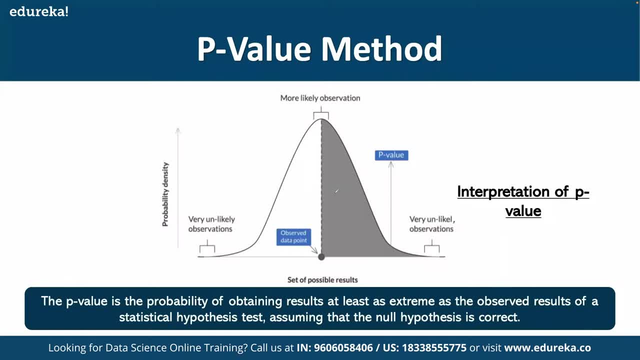 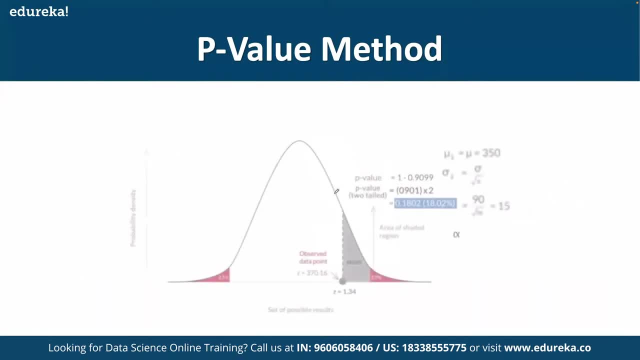 okay. so here, like it's the probability of obtaining the results at least as extreme as the observed of a statistical hypothesis test. so assuming that my null hypothesis is true of a statistical hypothesis test. so assuming that my null hypothesis is true, so with this we'll get the value of p and on the basis of the value of p value. 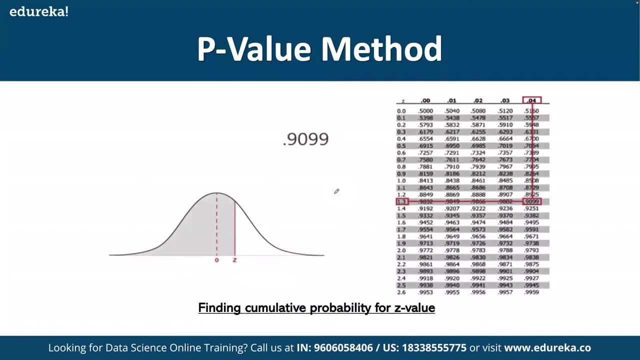 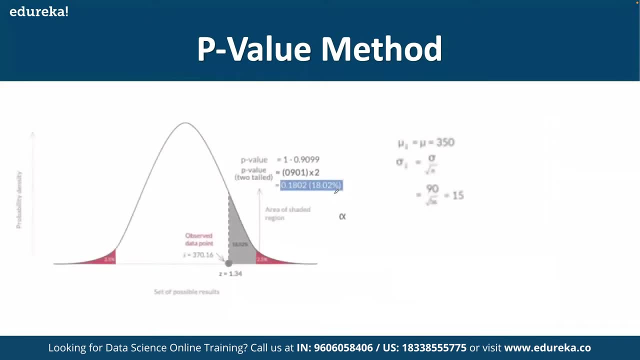 we are going to interpret whether it follows the null hypothesis and the alternate hypothesis. now, with the value of z we can get the value of p score and with the value of p score. so we will check whether it the, whether it with with the respective value of the value of p. 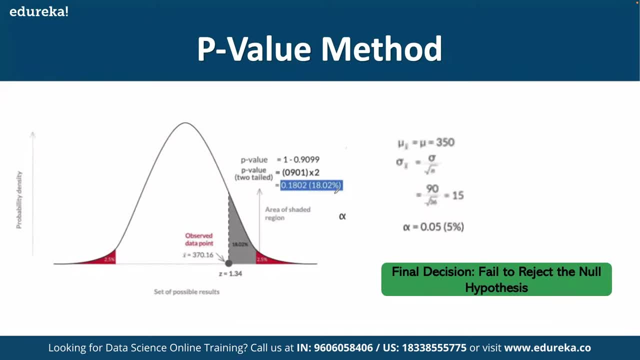 so, like the p value, whether it is less than 0.0 or greater than 0.05. based on this, we will either accept the null hypothesis or we are going to reject the null hypothesis. so that's the overall idea when it comes to the approach of 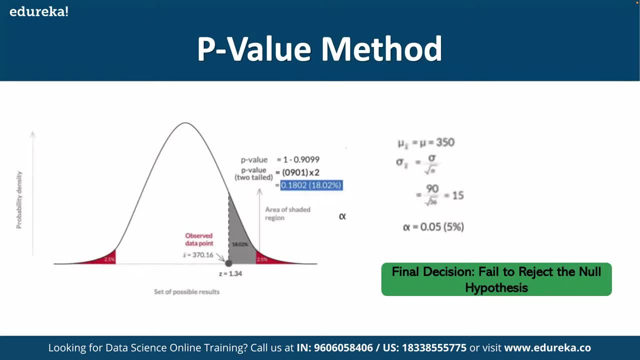 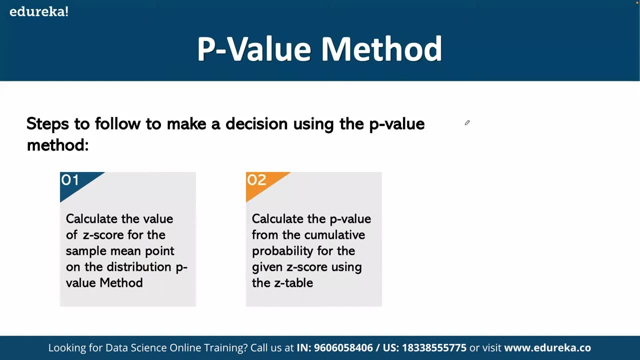 the p value method. so in case of p value method, the steps that we follow in this hypothesis testing are: first we'll calculate the value of z-score for the sample mean point on the distribution using the p-value method. Then we'll calculate the p-value. 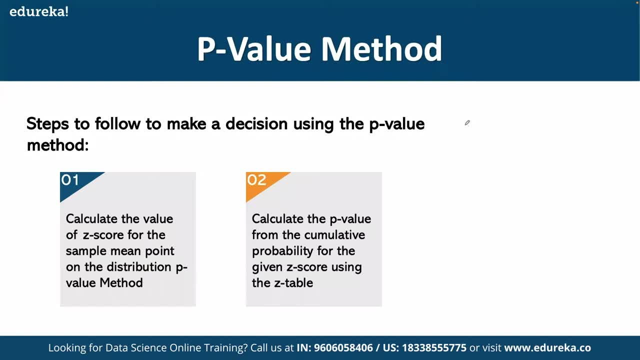 from the cumulative probability for the given z-score using the z-table, And this is followed by making a decision on the basis of p-value with respect to the given value of alpha. Okay, so these are the steps that we generally follow in order to make a decision using a p-value method. 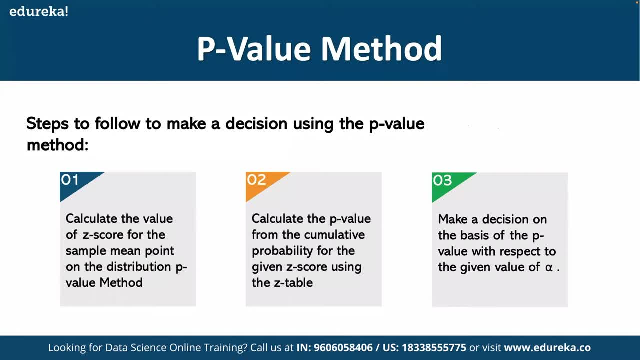 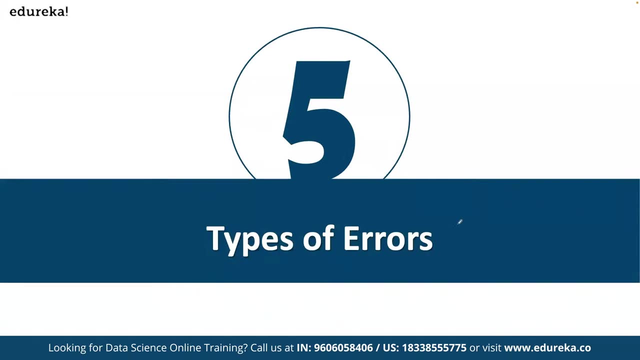 So you are now familiar with two methods. One method is called as the p-value method. The other method is the critical value method. Now that you're familiar about this, now let's go ahead and understand the types of errors that we have got. 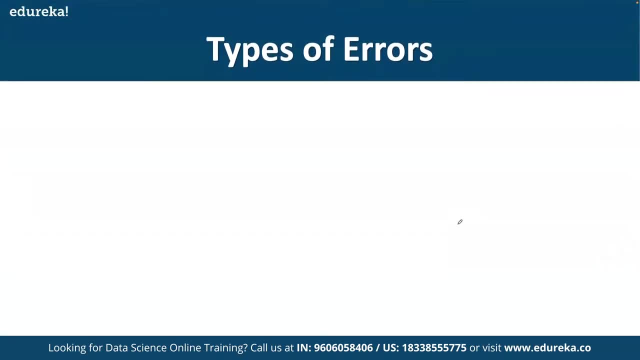 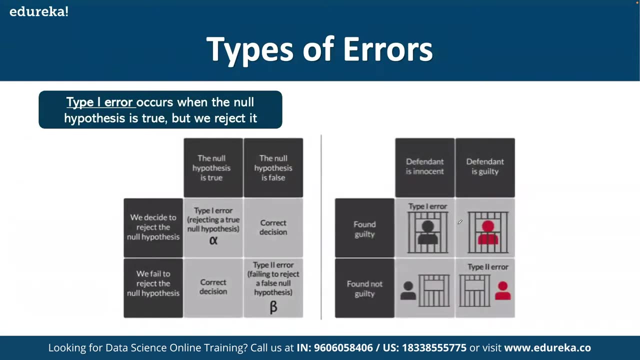 whenever we are performing the hypothesis testing, So during the hypothesis testing. so we have got type 1 error and the type 2 error. So in order to do that, to determine whether it belongs to a type 1 error or the type 2 error, 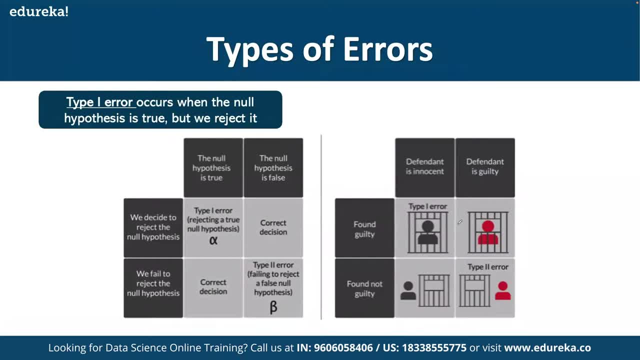 we find it with the help of the confusion matrix. So confusion matrix helps us to describe how my model is confused, in which scenarios my model is actually confused when it is performing the classification. So type 1 error means when the null hypothesis is true. 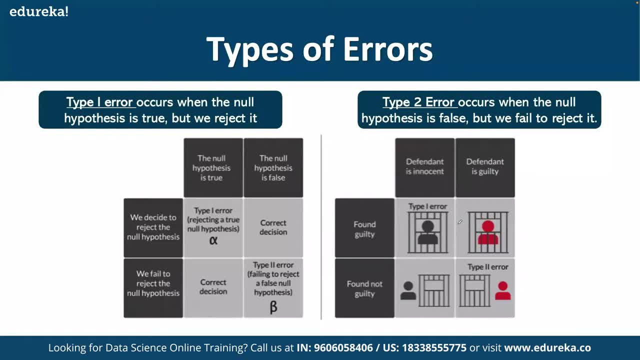 but we are rejecting the null hypothesis and going with the alternate hypothesis. So that is what we are doing. So that is a scenario where we call it as a type 1 error And we've got the type 2 error, And this would occur when the null hypothesis is false. 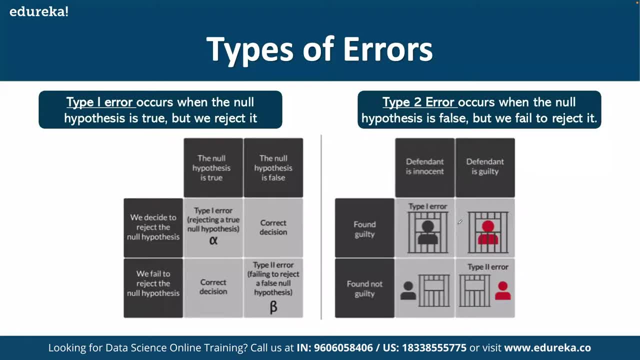 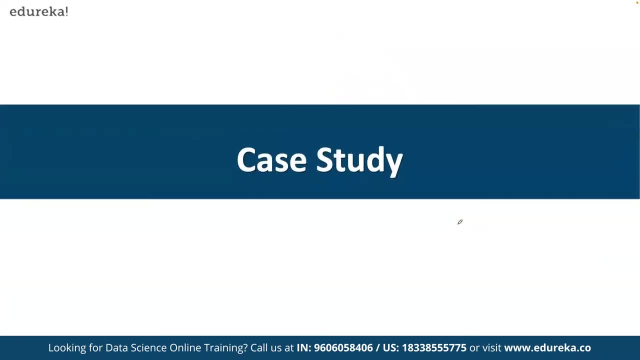 but we fail to reject it. So these are the two kinds of error that we generally come across while performing the hypothesis testing. Now, to get a better clarity on this, let's take up a case study. Now, in the scenario of case study, 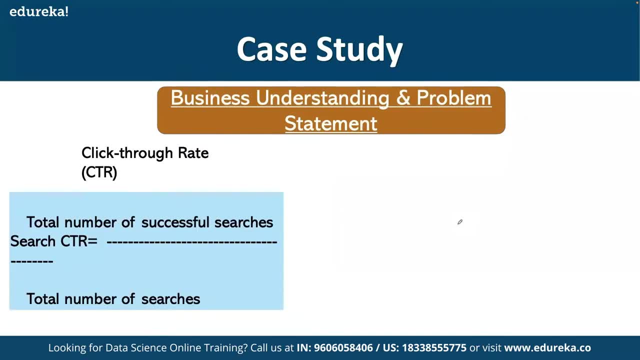 so let's say we've got the total number of success. successful search is given by CTR, which is nothing but the total number of searches. Now, as a data analyst at ScriptCard and the product like as a. now let's say, you are a data analyst. 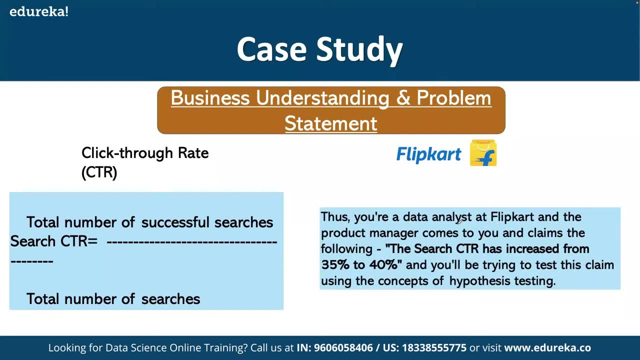 and the product manager comes to you and claims the following: that the search CTR has been increased from 35% to 40%. Now, this is what we are going to check, like here We are going to, we are going to test whether the claim 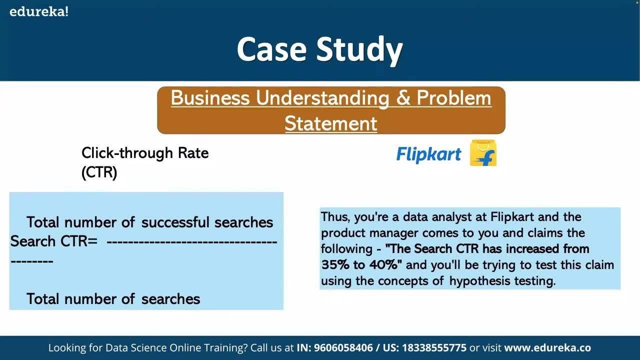 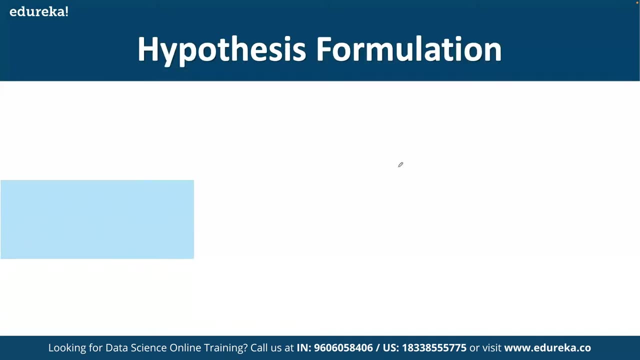 made by the product manager, whether it has, whether it is statistically valid from the given data or whether it is statistically invalid Now, in order to check that, you are going to perform the hypothesis testing. So the formulation of hypothesis testing is something like this: 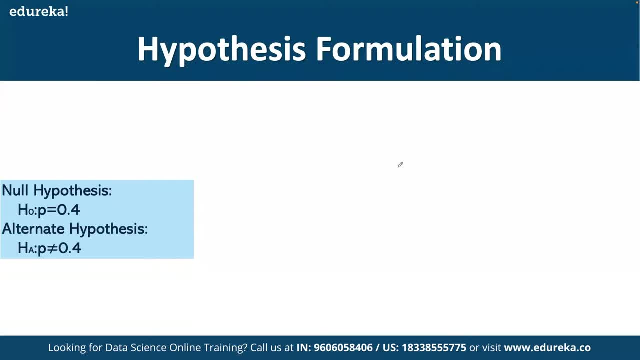 First you are going to define the null hypothesis and the alternate hypothesis. The null hypothesis says that okay, there's a 40% CTR. that is say that P is equal to is equal to 0.4.. And the alternate hypothesis is: P is not equal to 0.4.. 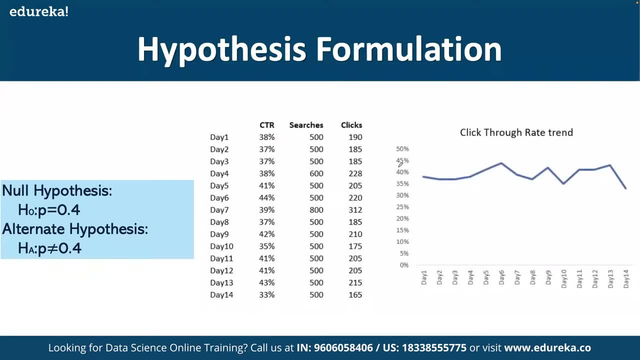 So first step is defining the null and the alternate hypothesis. So you are going to collect the data. Let's say you have got the data of CTR- okay- from the given data set and you've got the information about searches and the clicks. 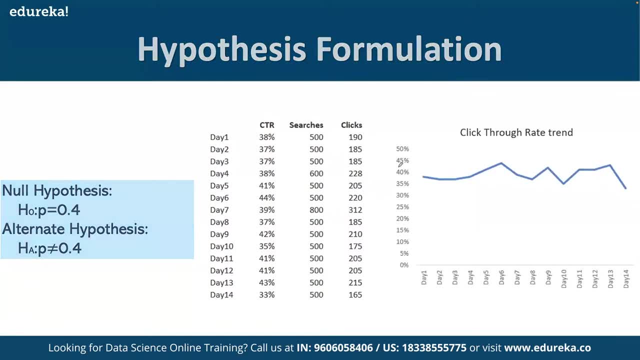 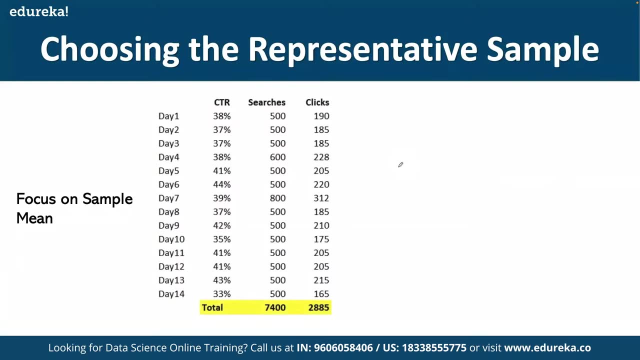 Okay, that is what you have got over here in this given data. Okay, now, once you have got the population from the sample you are going to collect, from the population you are going to collect a sample and you will focus on the sample mean. 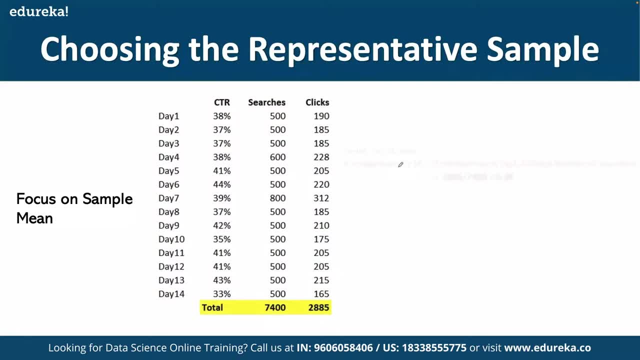 Here the sample mean, once you find it. so this is what we would get as an average CTR. So the average CTR is given by 0.39.. And the sample mean is 0.39.. And we have got the sample size as 7400.. 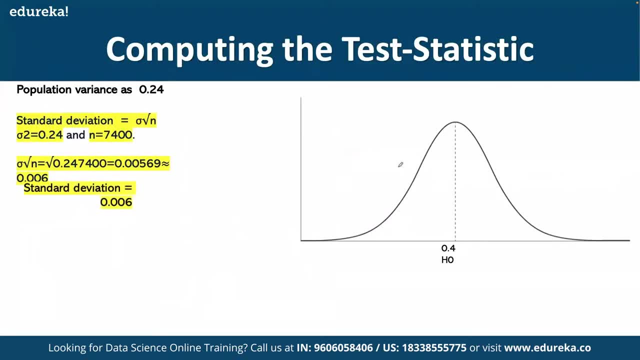 Okay, so with this information, we are going to compute. we are going to compute the test statistic, So I'll calculate the population variance, And once I compute my population variance, so I'll get the standard deviation. So, with these values, 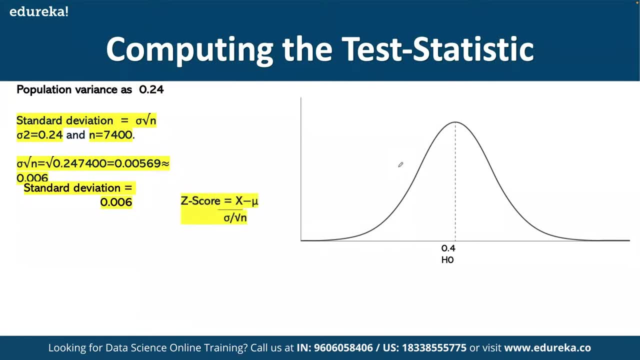 we'll get the respective Z-score. Z-score is given by X minus mu, divided by standard deviation of a sample. Okay now, once we have done this activity, so we'll get the respective test statistic. In this scenario, we'll get the Z-score. 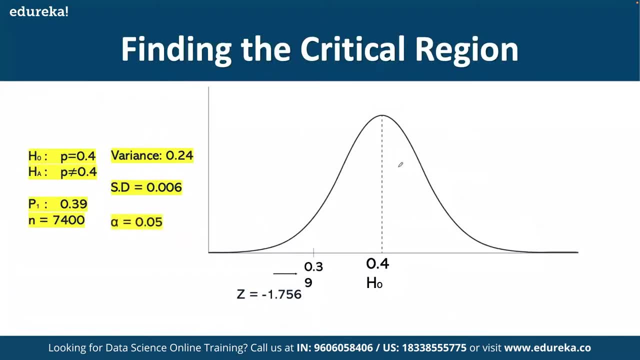 Now, once I have the Z-score, I'm going to check the scenario. okay, with the alpha as 0.05.. So I'm going to check for a given data, Okay, so what exactly will be its respective P-value? Now, with the value of P, 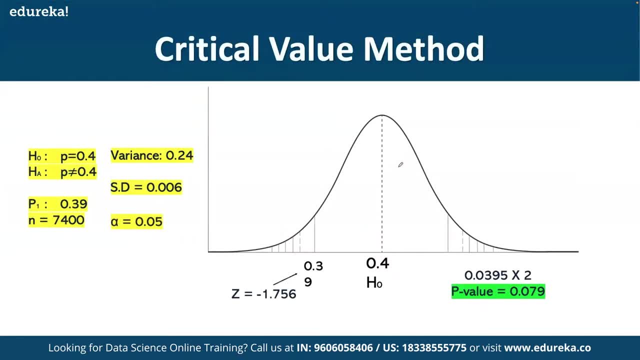 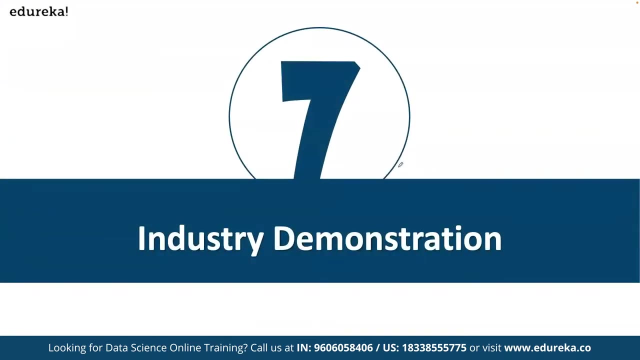 I'm going to decide whether it follows the null hypothesis or whether it follows the alternate hypothesis. Okay, so that's the way in which that we are going to interpret the results. So, now that you have seen how we can perform the hypothesis testing, 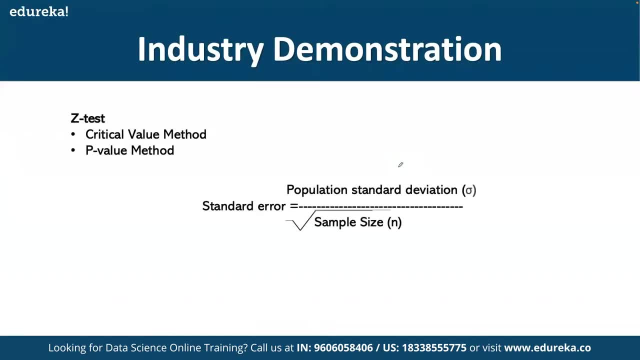 let's take up an example. So here the Z-test is given by critical. like in case of Z-test we can do by two methods. One is critical value method and the other one is a P-value method. So while calculation of Z-value 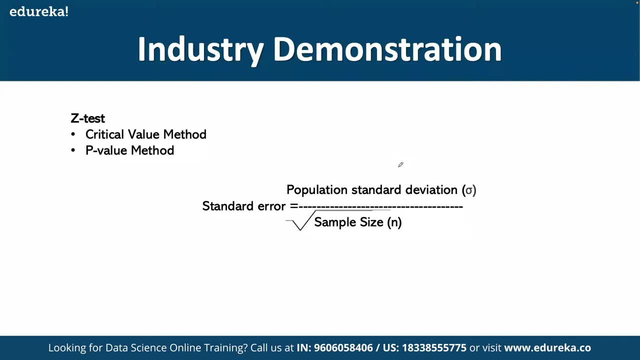 we'll be finding the standard error, which is given by population standard deviation divided by square root of sample. So here we have the sample size and apart from that we've got the T-test and the T-distribution. So, coming to the T-distribution, 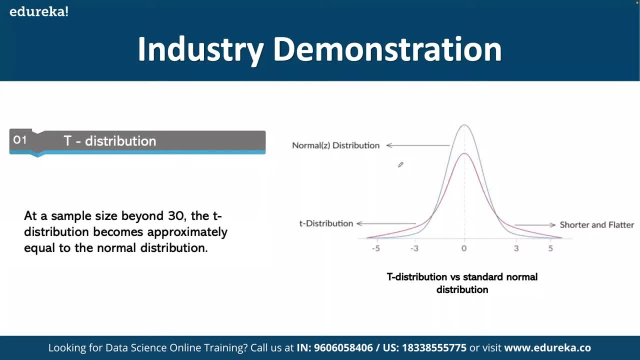 so this is a diagram which describes the T-distribution. Okay, so T-distribution are little bit shorter and flatter, So at the sample size beyond 30, so the T-distribution becomes approximately equal to the normal distribution. Okay, this here. 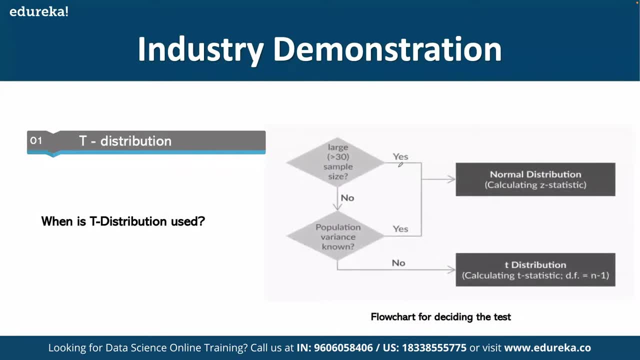 we use this T-distribution. we are calculating the T-statistic with D, like with degrees of freedom. is N minus one. Okay, this is how we decide whether to use the T-distribution or normal distribution. So if I've got a large sample, 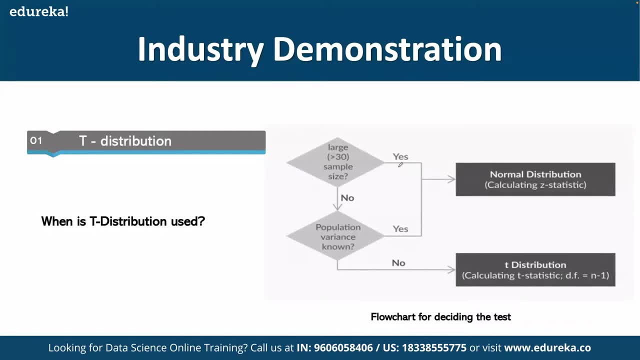 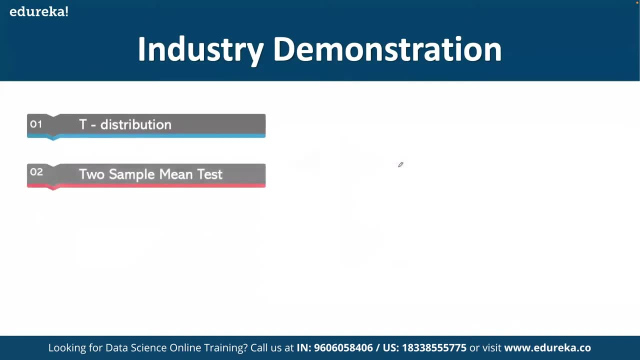 then I'll use the normal distribution. If I've got a very small samples and population variance is not known, then in such scenarios we use the T-distribution And there is something called as two sample mean test. Now, in this, two sample mean test. 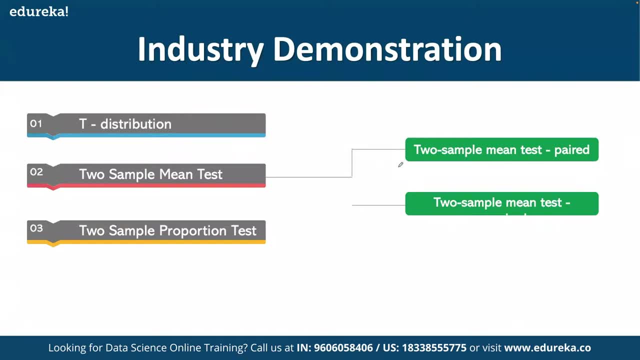 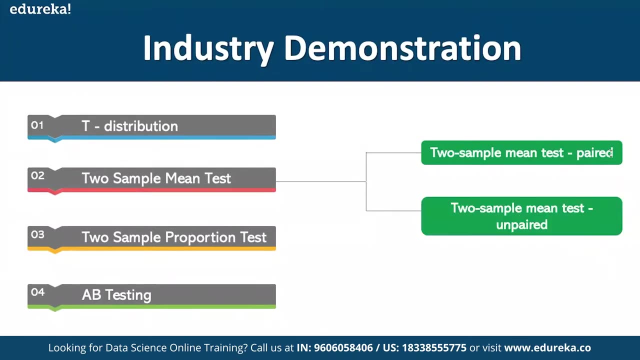 so here, under this, two sample mean test. we've got to like two sample pair test, Okay, and two sample independent test. Let me show you what it would mean. So here like two sample test under this we've got paired and we've got unpaired or an independent. 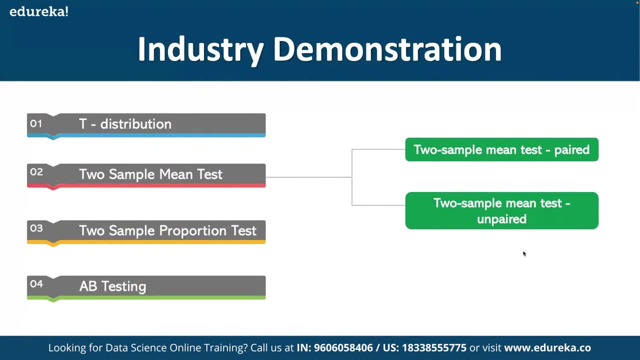 So this is another kind of testing that we have got, and we've got two sample proportion Test and the AB test. So these are the various hypothesis test that are available in statistics which we can apply it on a data set. All right team now in order to implement this in Python programming language. 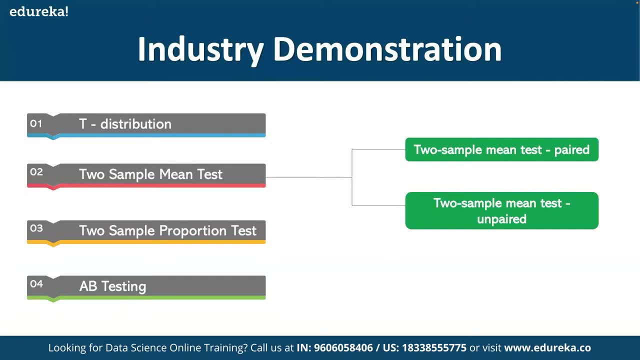 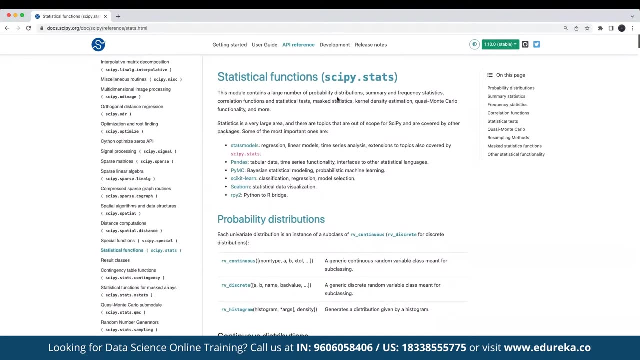 we can make use of various functions which are available inside the scipy library and you from the scipy library. There's a specific module called stats. Let me show you the official documentation of the same. So this is the official documentation page of scipy dot stats here. 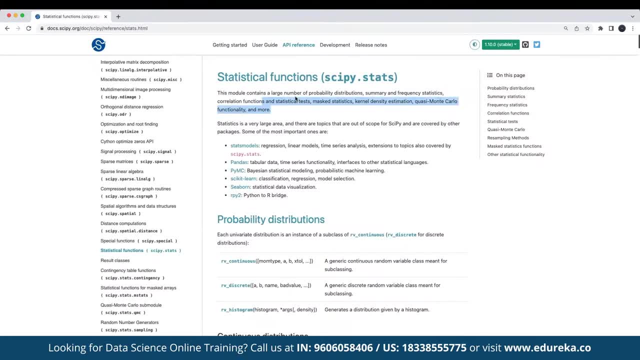 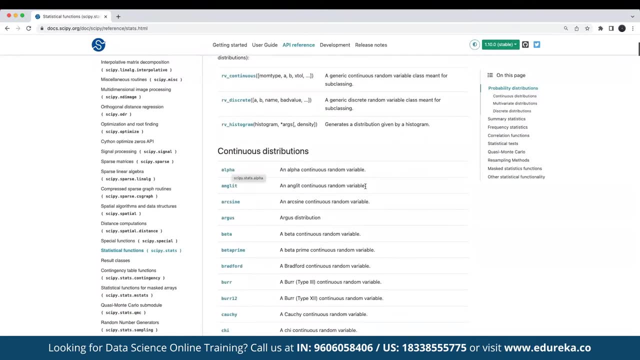 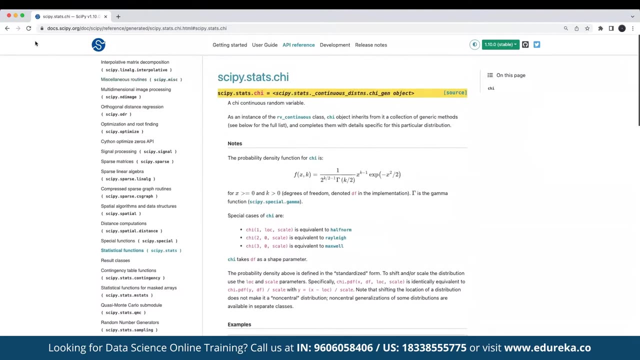 We've got various statistical functions under the scipy dot stats. So, like various information, we can find an alpha continuous variable. See, you can excuse me If I want to find the chi value. we can actually get it using the chi function. So you can check out the various. 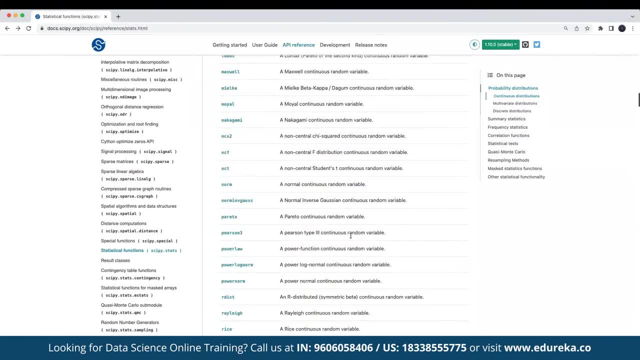 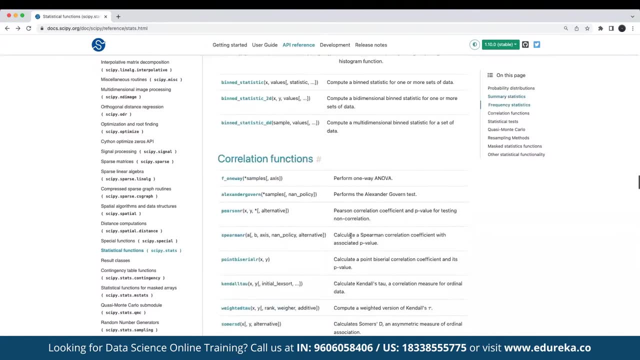 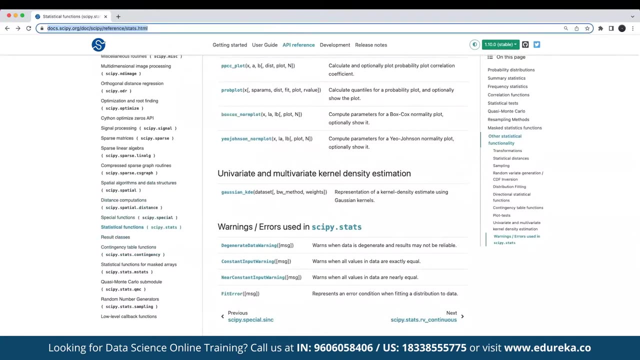 functions that are available in this scipy Dot stats. Okay, so you can also check as well And learn about, learn more about the various statistical functions that we have caught with us under this scipy dot stats. All right, team. So with this we come to the end of today's session. 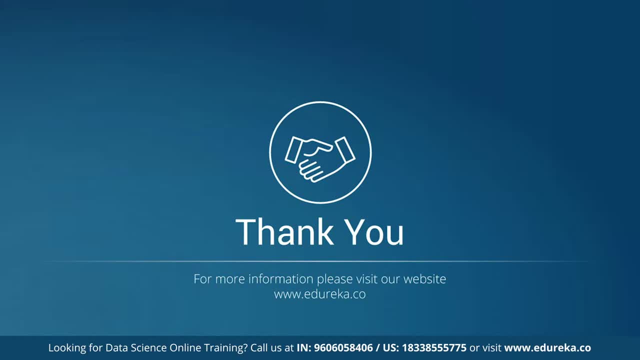 So, as part of a learning journey, today we have looked into what it means by hypothesis testing and how do we perform the hypothesis testing. So thanks again for joining in and I'll see you next time. Take care, everyone, Bye, Bye.